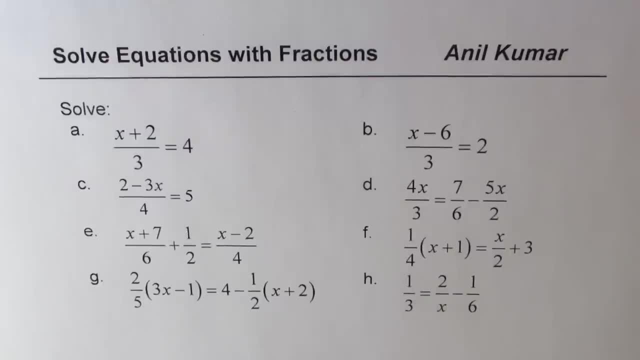 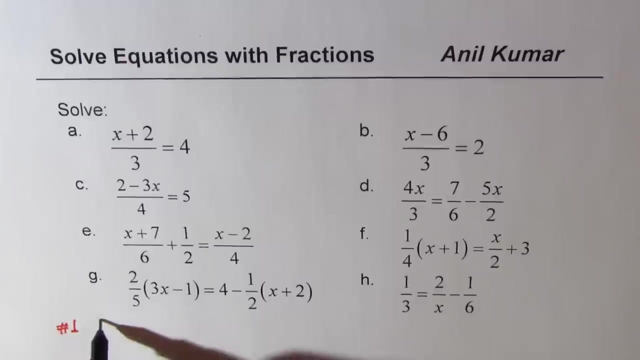 you to pause the video, copy these questions and then we are going to take them one by one. I am going to use two strategies here to solve all these questions. Let me call strategy one as cross multiplication and strategy two as get rid of fractions. Now, cross multiplication also helps to get rid of fractions. Let's say the number is: 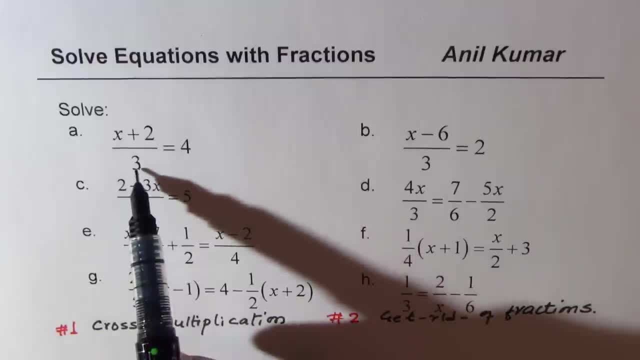 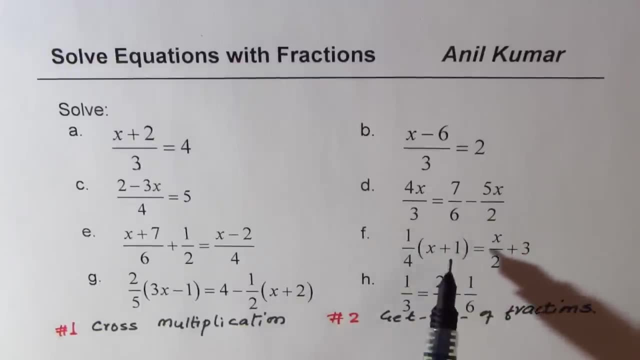 3 here. We'll just take it on the other side, So we'll get rid of 3 from the left side. Now, sometimes what happens is we have different numbers right. For example, here we have three terms Here how do we get rid of fractions? So in this case we'll look for the LCM. 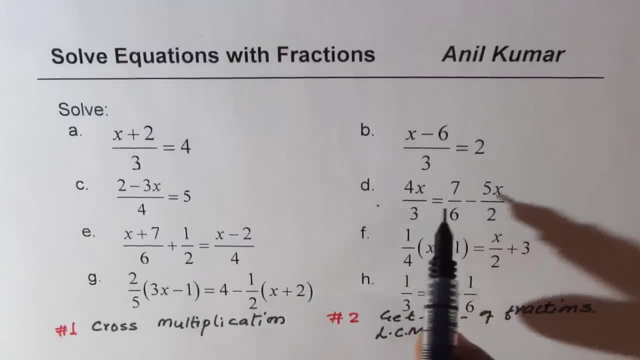 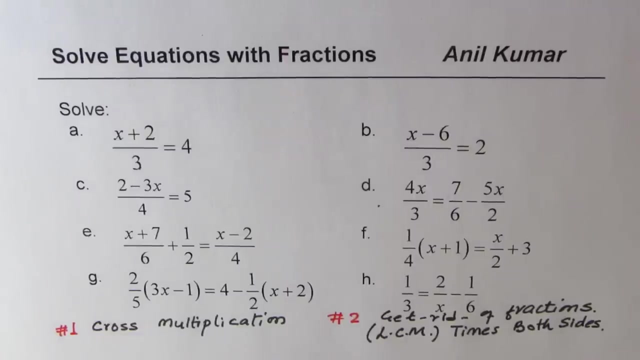 lowest common multiple. We'll multiply both sides by lowest common multiple. So the strategy will be LCM times both sides, And then we'll solve as a linear equation without fractions. So I hope the strategy is absolutely clear. Now let's apply this strategy to all these. 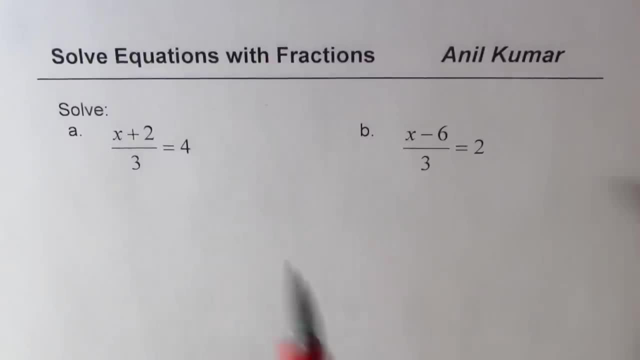 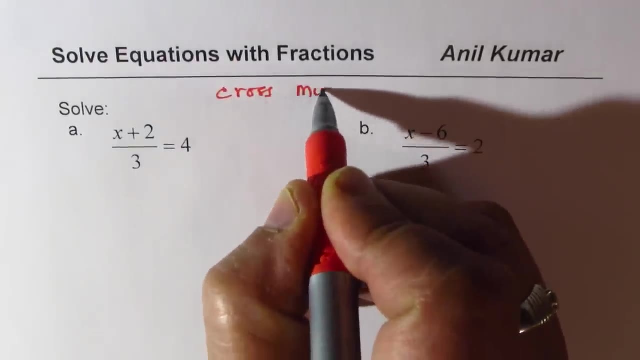 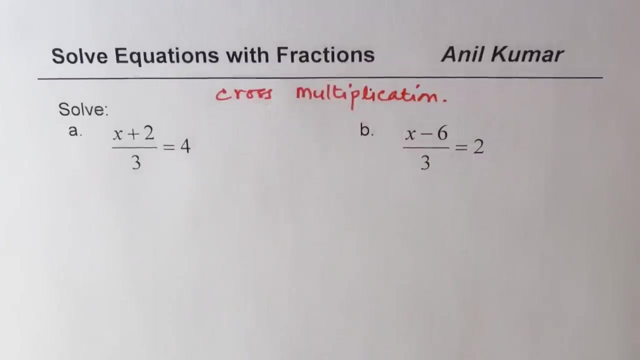 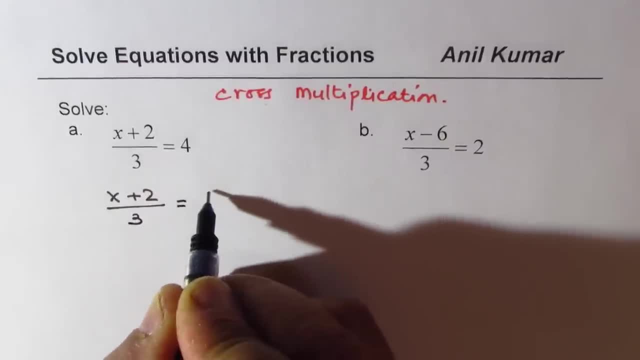 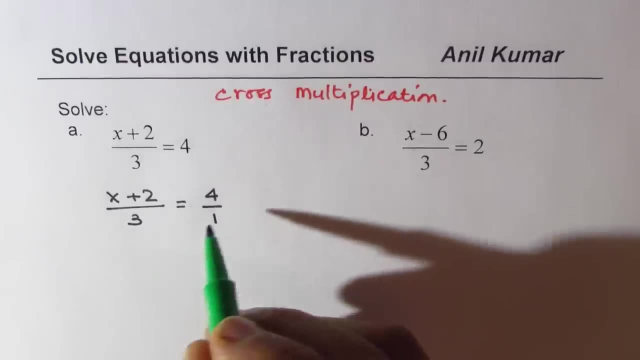 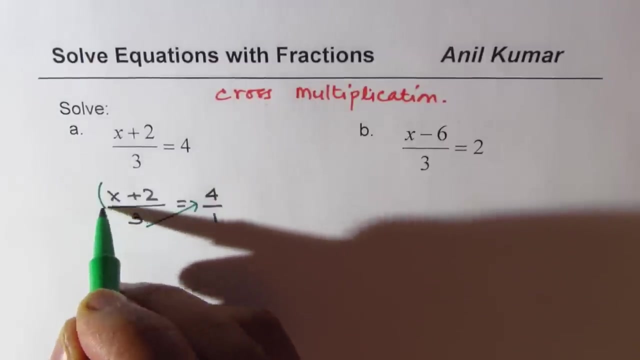 y, y over x plus 2 over 3 equals to 4 over nothing, So think we have 1 here. So cross multiplication means this 3 gets multiplied with the term on the right side And this term, the whole term, gets multiplied. 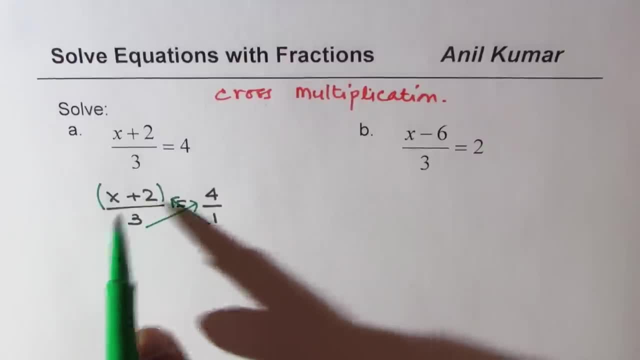 by 1.. You get an idea right. That means it remains kind of same. That's what we mean. So cross multiplication: We're left with x plus 2,. employer: The unit value divided by x. beer one divided by x, even green plus x plus two. meat minus 구28.. Here you know. 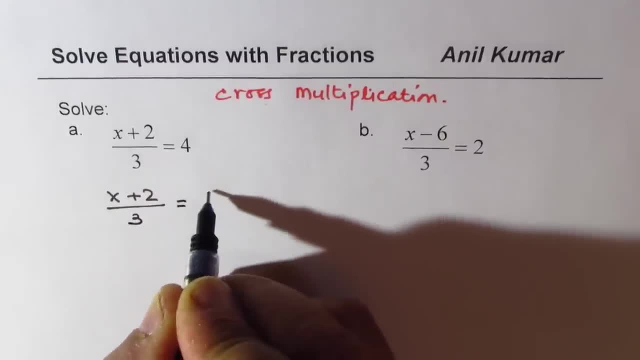 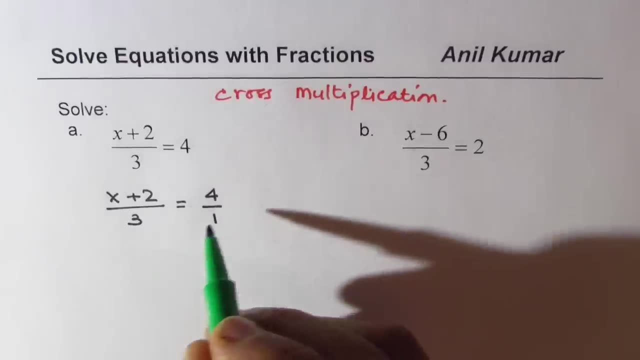 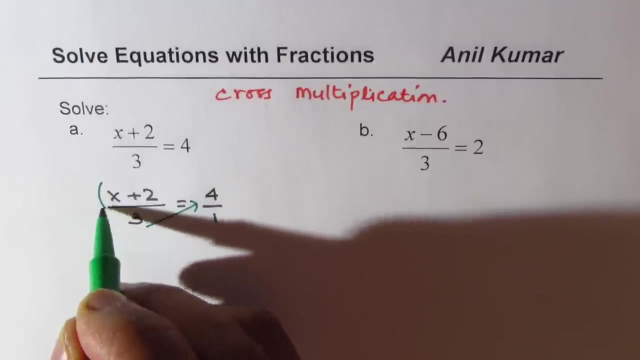 x plus two over three equals to four over nothing, So think we have one here. So cross multiplication means this three gets multiplied with the term on the right side and this term, the whole term, gets multiplied by one. You get an idea, right? That means 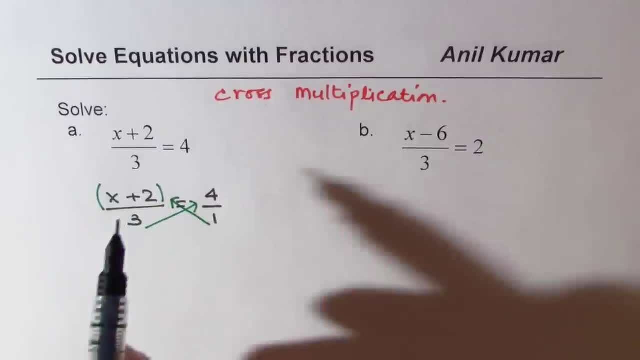 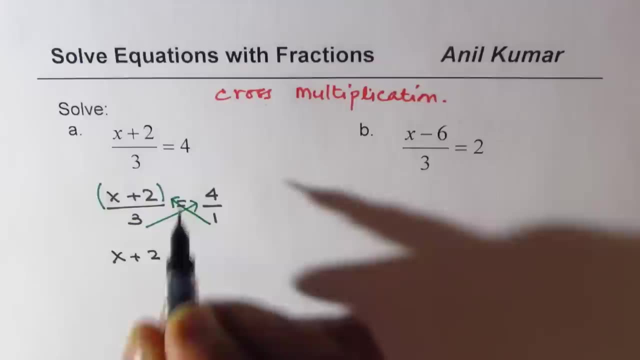 it remains kind of same. That's what we mean, So cross multiplication. we are left with x plus two over three. That's what we mean, So cross multiplication. we are left with on the left side and on the right side we get 4 times 3 or 3 times 4, one of the 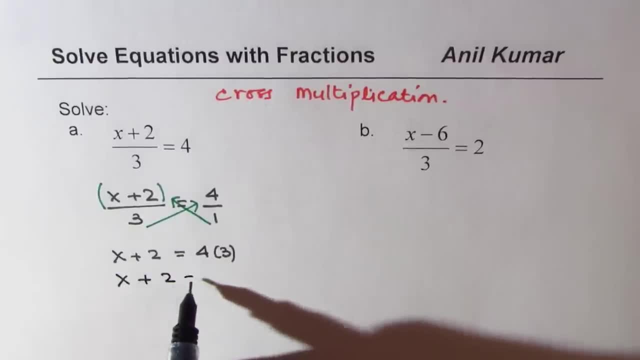 same thing. so what we have here is X plus 2 equals to 12, and now this is, without fractions, easy to solve. X equals to 12 minus 2, which is 10. so we get X equals to 10. some of you can check the answer by placing 10. what do we get we? 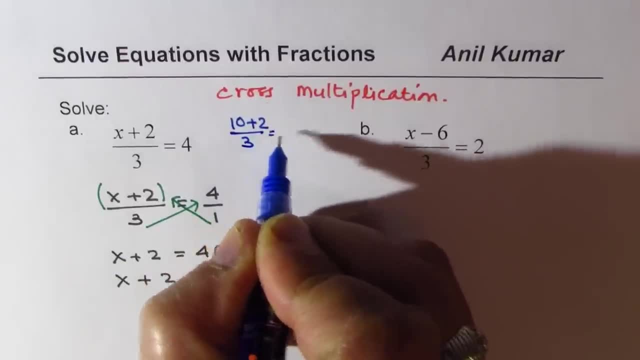 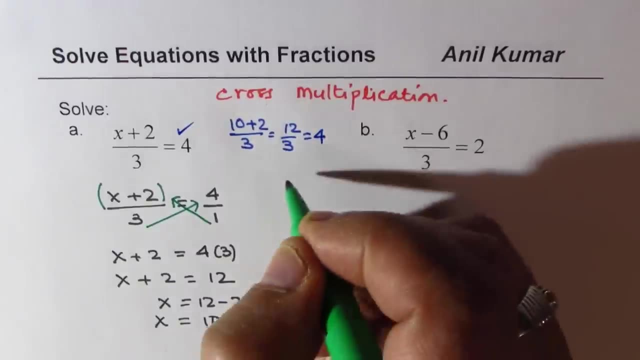 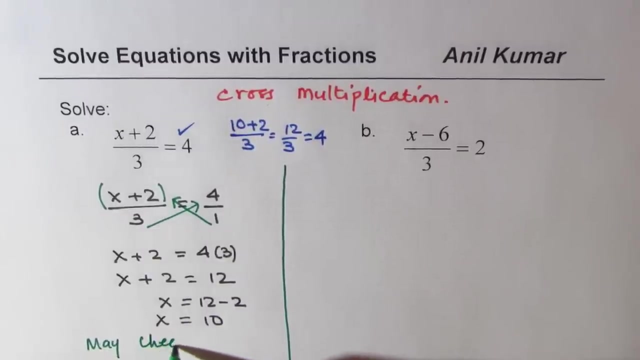 get 10 plus 2 over 3, which is 12 over 3, which is indeed 4. so that works perfect. so you may or may not check for the time being, but it's a good practice so you may check, okay. so I think the technique is absolutely clear. let's apply it once. 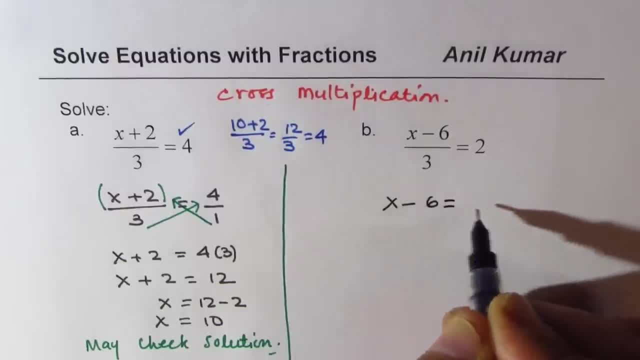 again. so we get what we get: X minus 6 equals to 12 plus 2, equals to 12 minus 3, which is 12 over 3, which is 12 over 3, which is to 2 times 3. so that is x minus 6 equals to 6. x is equals to 6 plus 6, so x is equals to 12. 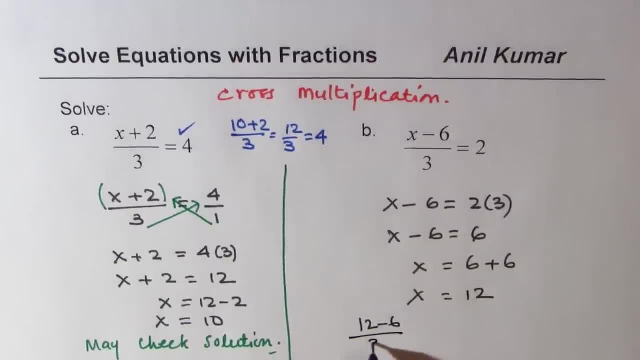 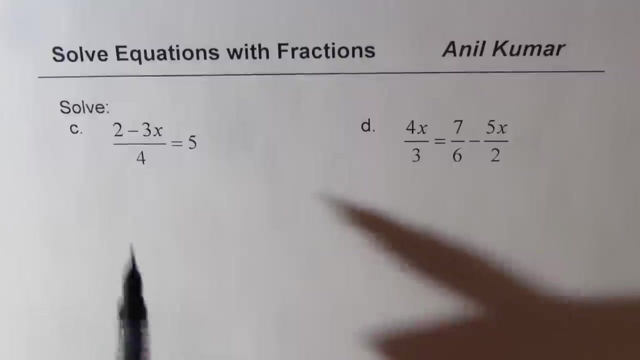 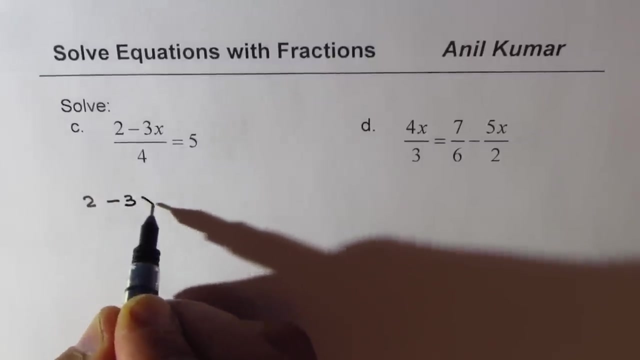 and you can check your answer: 12 minus 6 over 3 is 6 over 3, which is indeed 2. so that's what you expected, correct? okay, so we have another similar kind of equation now. here we'll apply both the techniques. so this one i think now you can do easily. we can write this as: 2 minus 3 x equals to: 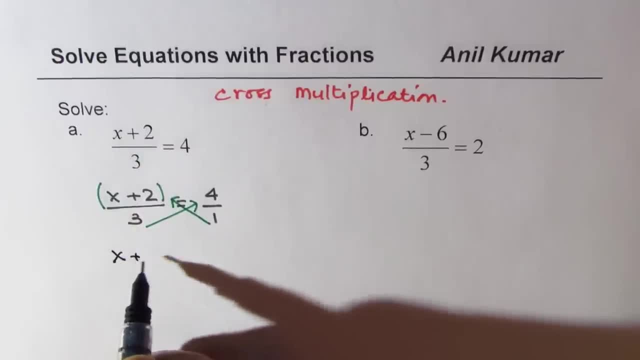 the answer is sum, Understand It's integral and the net value linearには principle. We'll see this written directly afterこちら, Because we're using this function 2 on the left side and on the right side we get 4 times 3 or 3 times 4, one and the same. 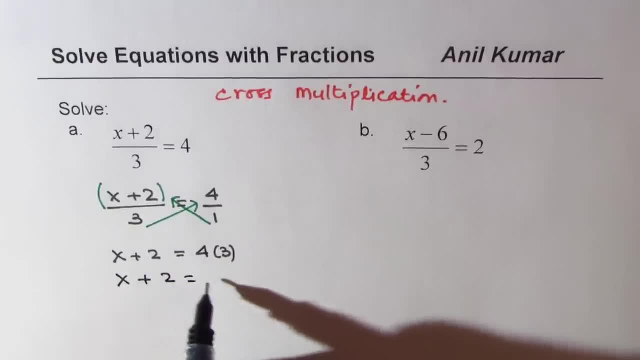 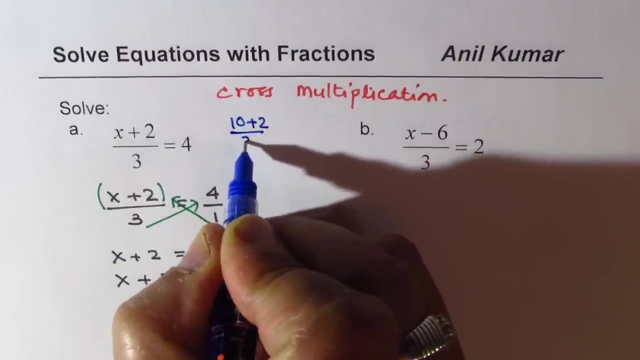 thing. so what we have here is x plus 2 equals to 12, and now this is, without fractions, easy to solve. x equals to 12 minus 2, which is 10. so we get x equals to 10. some of you can check the answer by placing 10. what do we get? we get 10 plus 2 over 3, which is 12 over 3 which. 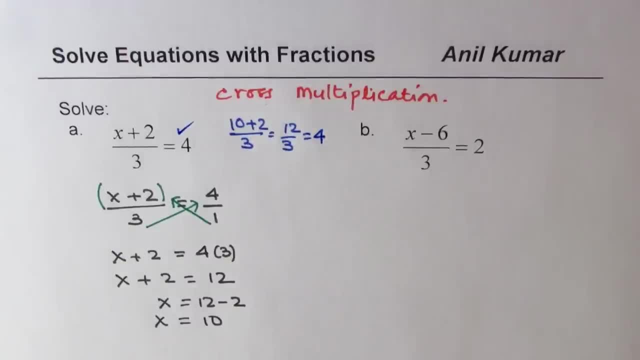 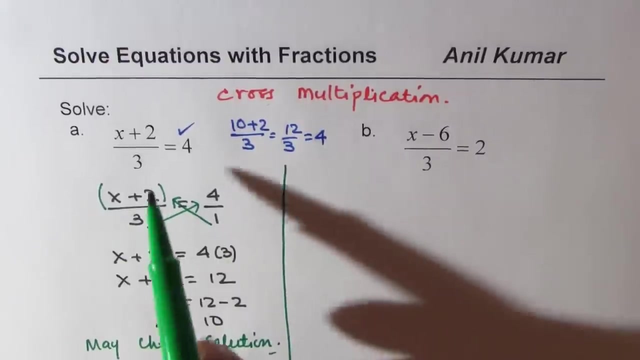 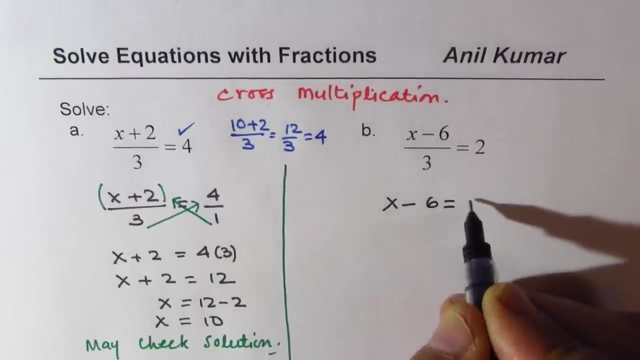 is indeed 4, so that works perfect. so you may or may not check for the time being, but it's a good practice so you may check, ok. so I think the technique is absolutely clear. let's apply it once again. so we get what we get. X minus 6 equals to 2. 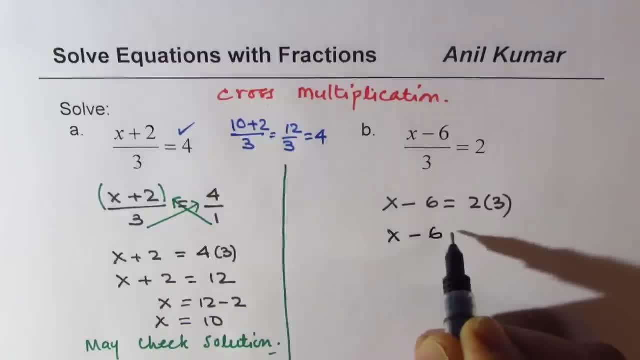 times 3. so that is X minus 6 equals to 6. X is equals to 6 plus 6, so X is equals to 12, and you can check your answer. 12 minus 6 over 3 is 6 over 3, which is. 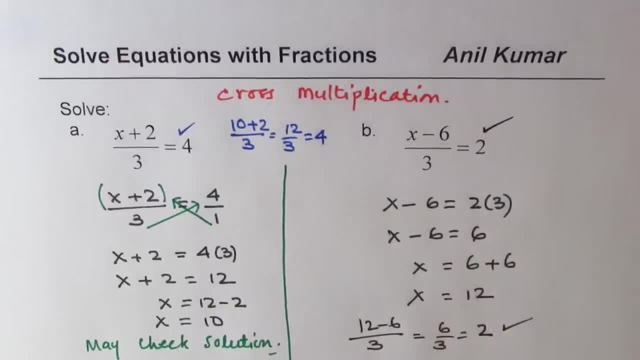 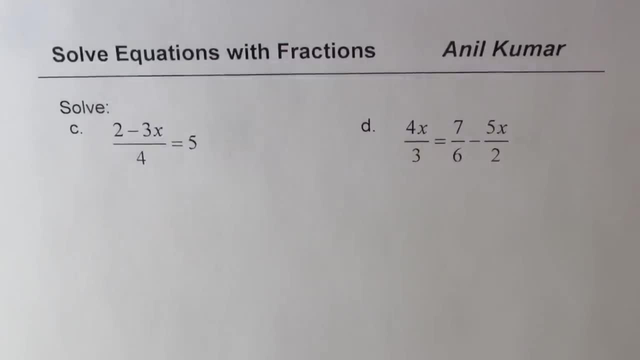 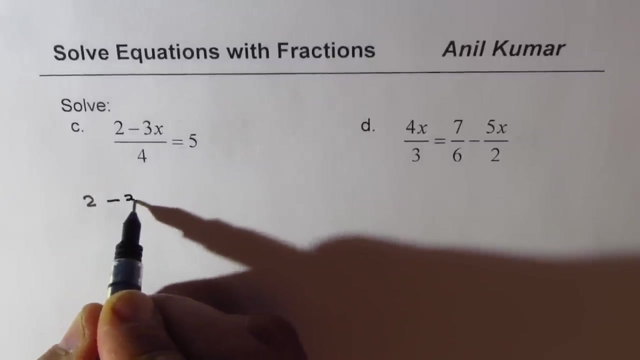 indeed 2, so that's what you expected, yeah, okay. so we have another similar kind of equation now. here we'll apply both the techniques, so this one I think now you can do easily. we can write this as: who minus 3x equals to 4 times 5, so we have 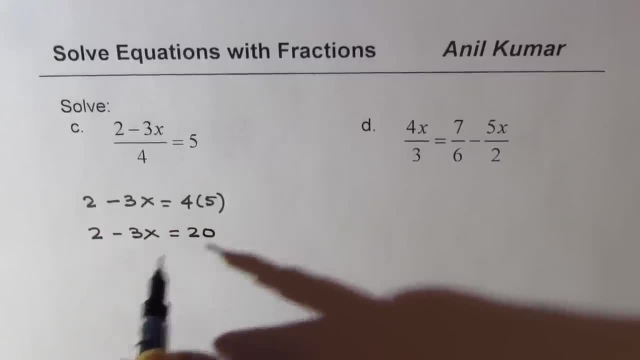 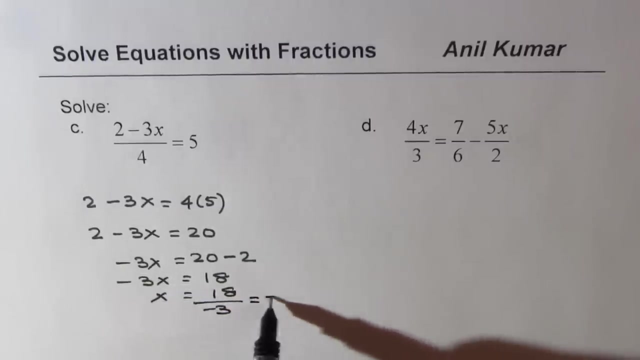 2 minus 3x equals to 20. minus 3x equals to 20 minus 2, so minus 3x is equal to 18. x is 18 divided by minus 3, which is minus 6, so we get x equals to minus 6. perfect. next one now here, what we see is that we see three different term. 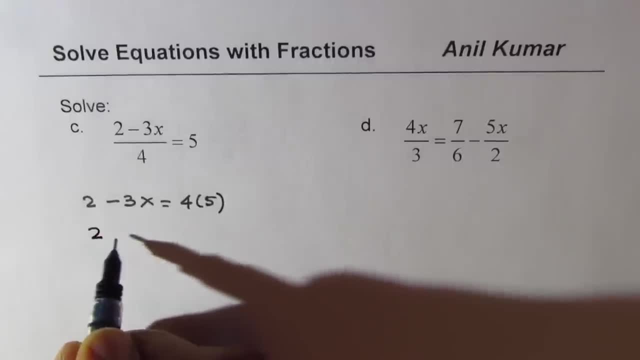 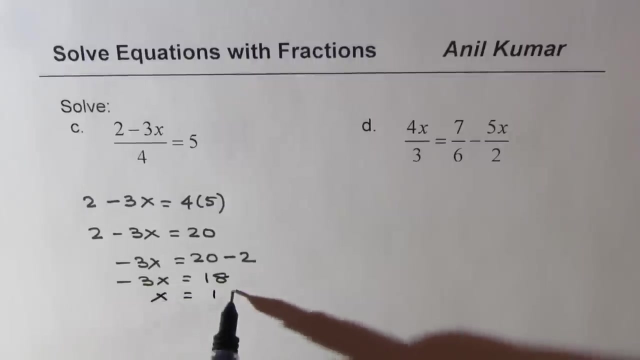 4 times 5, so we have 2 minus 3 x equals to 20, minus 3 x equals to 20 minus 2. so minus 3 x is equal to 18. x is 18 divided by minus 3, which is minus 6. 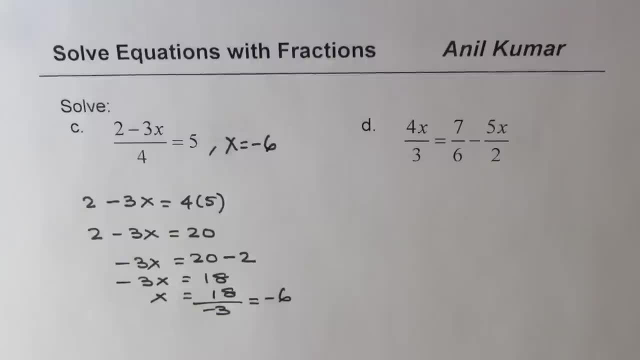 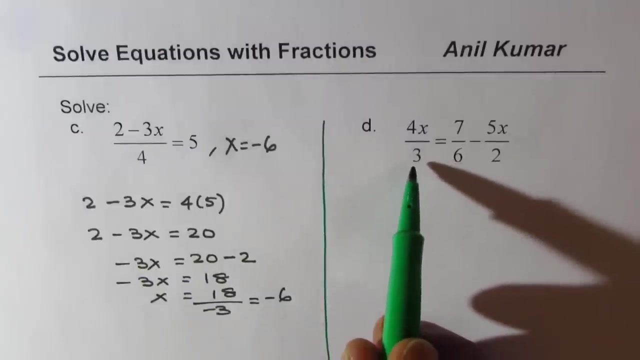 so. So we get x equals to minus 6, perfect. Next one: now here, what we see is that we see three different terms. so this technique is not going to work. We have to find the lowest common multiple. so, in this case, what is the LCM? so we are. 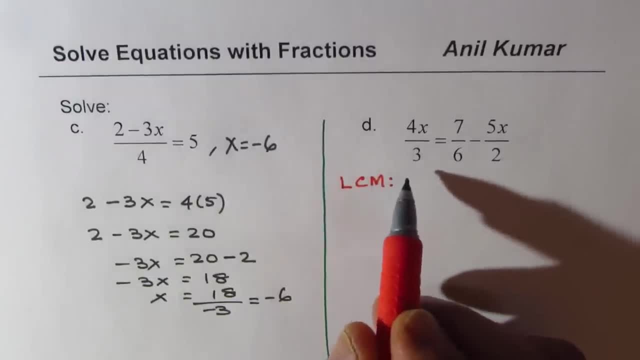 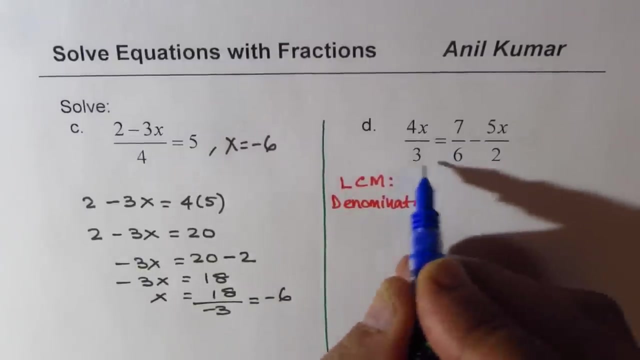 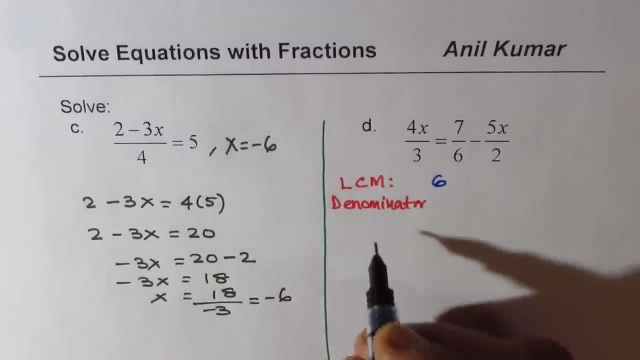 using the second strategy, we are finding lowest common multiple for denominator, so this is for denominator, So 3,, 6 and 2, the lowest common denominator is 6, so we are going to multiply each term by 6, right, so let's rewrite this. 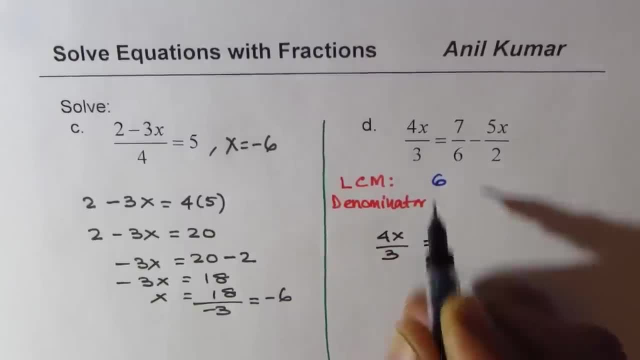 So we get 4x over 3, equals to: the equation is 7 over 6 minus 5x over 2, we are going to multiply each term. So we get 4x over 3, equals to: the equation is 7 over 6 minus 5x over 2, we are going. 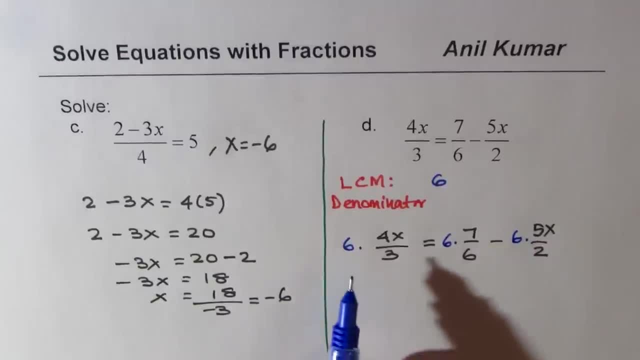 to multiply each term by 6 on both the sides. Do you see this? Now, since you do the same operation on both sides, you don't change the equation, but you could simplify it. so when you do so, you could get rid of fraction. that's the. 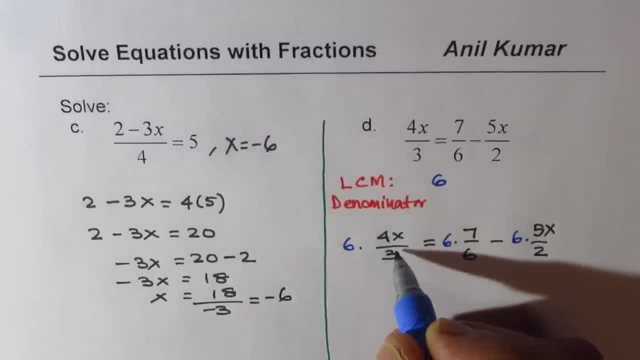 whole idea right. so here 3 goes two times, 6 one time, and that goes three times. so basically you get linear equation without fractions. 4 times 2 is 8, so I can write this as 8x. 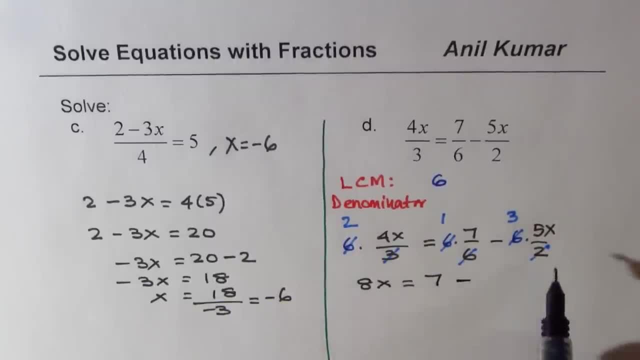 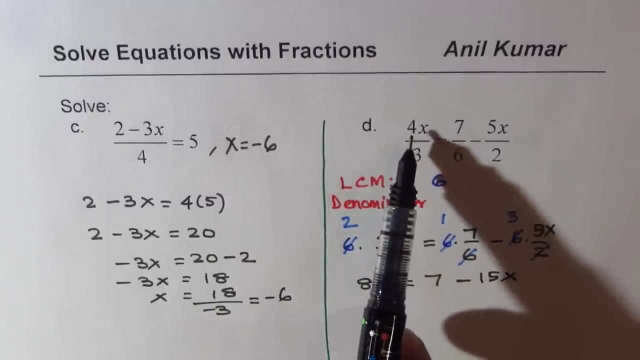 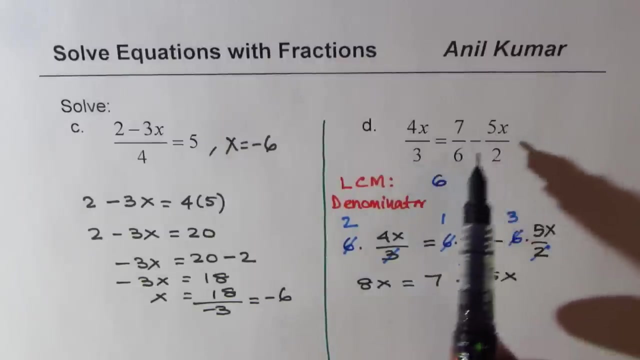 equals to 7 minus 3 times 5, 15x correct. So 4 gets multiplied by 2, we get 8x, 7 remains as such and 5 gets multiplied by 3, LCD also, we call lowest common denominator, so we will also call this lowest common denominator. 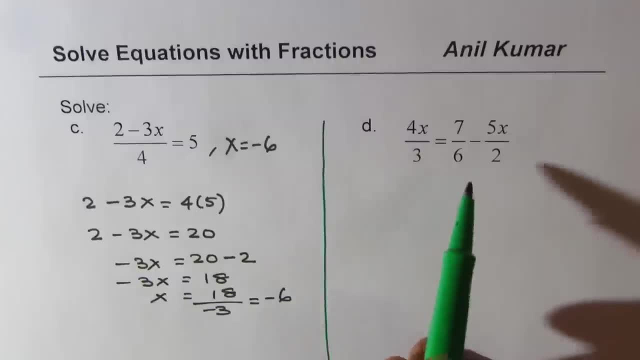 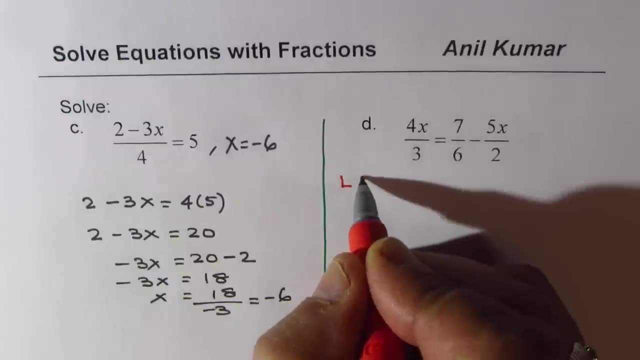 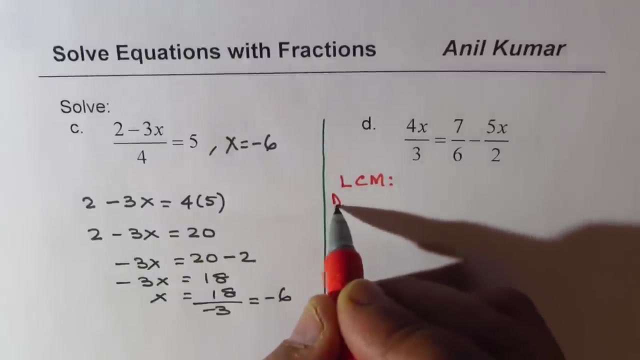 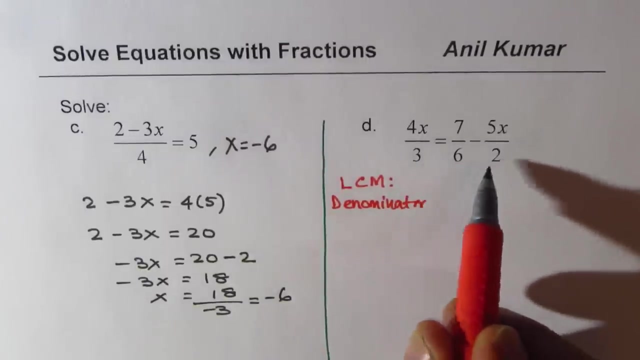 so this technique is not going to work. we have to find the lowest common multiple. so in this case, what is the lcm? so we are using the second strategy. we are finding lowest common multiple for denominator. so this is for denominator. so three, six and two, the lowest common denominator is six. 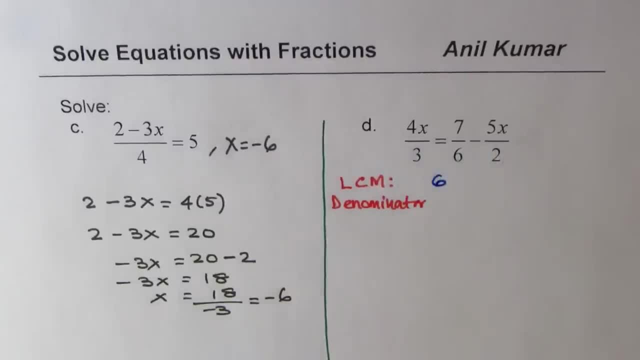 so if we nightmare is equal to one, so we are saying that. okay, this is for denominator, so we are again using the same chart. we are also doing OK, so in this case we have to. So we are going to multiply each term by 6, right? 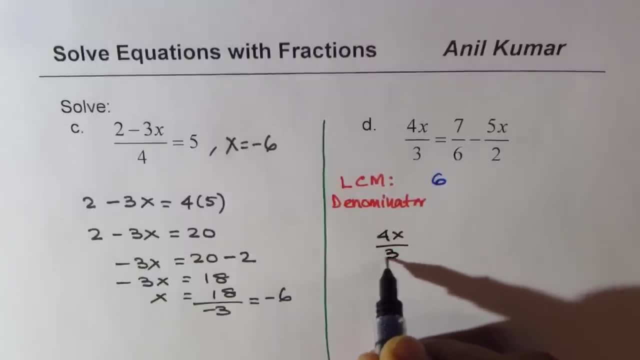 So let's rewrite this, So we get: 4x over 3 equals to: the equation is 7 over 6, minus 5x over 2.. We are going to multiply each term by 6, on both the sides. Do you see this? 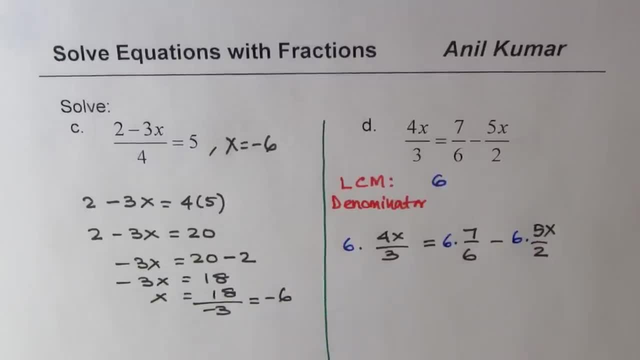 Now, since you do the same operation on both sides, you don't change the equation, But you could simplify it. So when you do so, you could get rid of fraction. That's the whole idea, right? So here, 3 goes 2 times, 6 one time, and that goes 3 times. 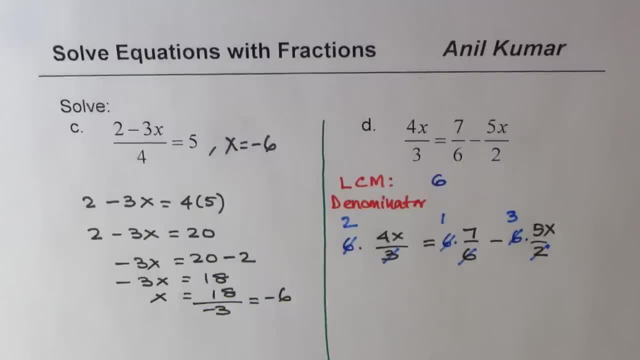 So basically you get linear equation without fractions: 4 times 2 is 8.. So I write this as 8x equals to 7 minus 3 times 5, 15x Correct. So 4 gets multiplied by 2.. 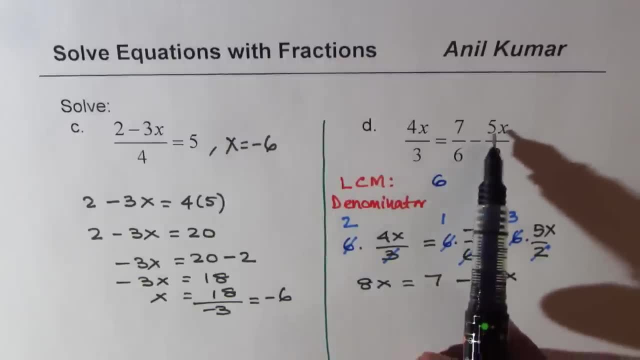 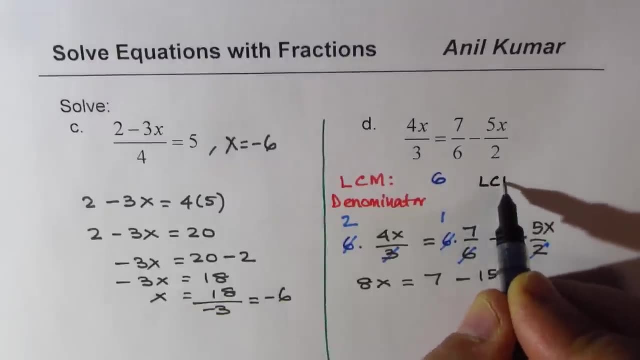 We get 8x. 7 remains as such and 5 gets multiplied by 3.. LCD also we call lowest common denominator. So we also call this lowest common denominator And you get a linear equation. Now it is simpler to solve. 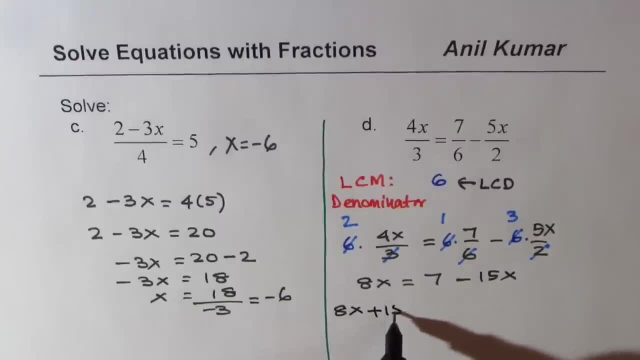 Bring it to one side: 8x plus 15x Equals to 7, and when you add this, 8 plus 5 is 13,. so you get 23x equals to 7,, so x is equals to 7 over 23.. 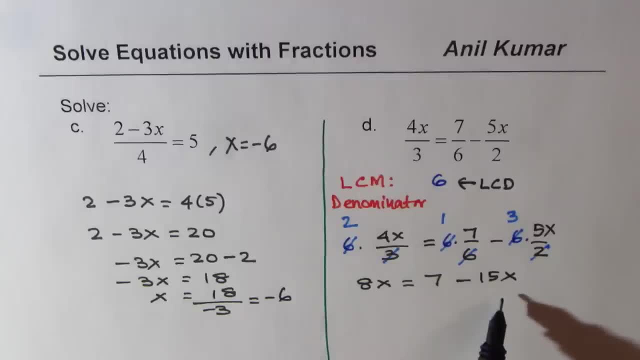 and you get a linear equation. Now it is simpler to solve. bring it to one side: 8x plus 15x equals to 7, and when you add this, 8 plus 5 is 13,. so you get 23x equals to 7, so x is equals to 7 over 23,, so that 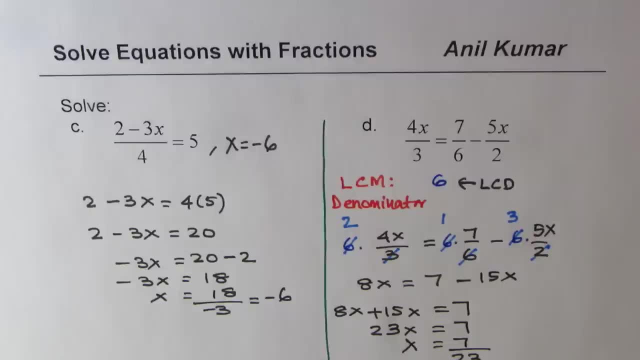 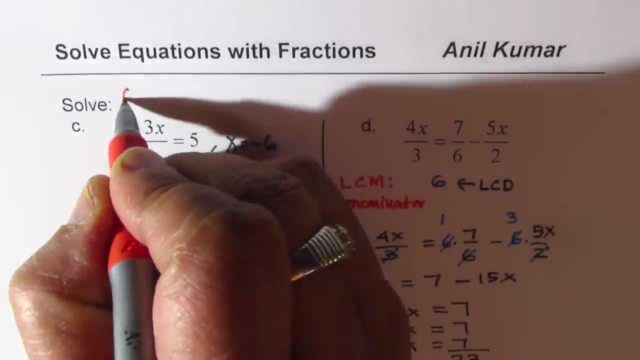 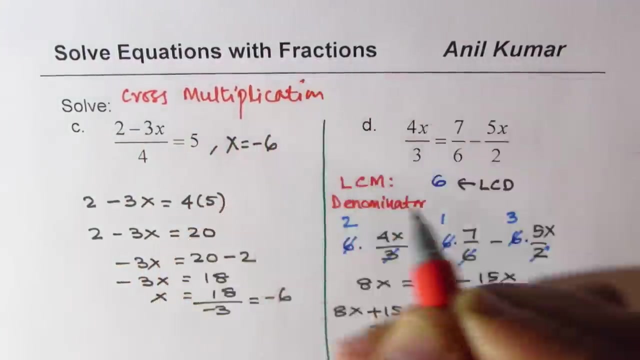 becomes the solution for the given equation. So I hope these steps are absolutely useful, Clear. So in this page we have seen both the techniques here. we did cross multiplication and then in D we found the lowest common denominator, which is actually the lowest common multiple. 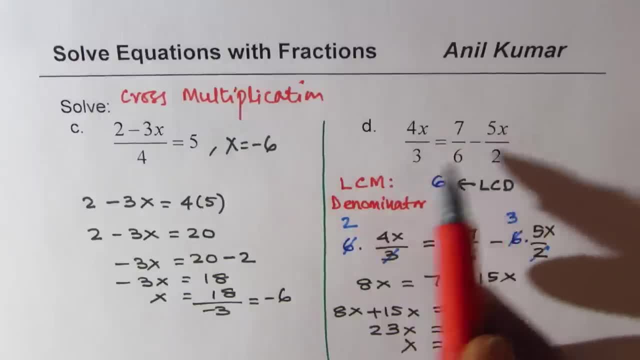 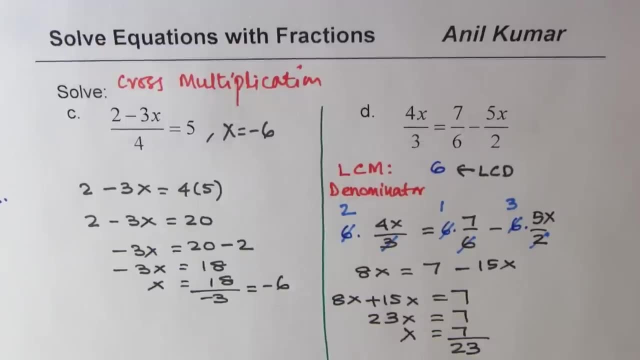 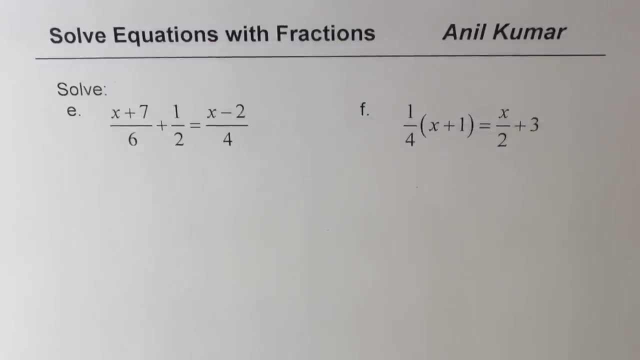 of the denominators. multiplying the same gets rid of the denominator and then you can solve as shown here. So I hope the strategy is absolutely clear. Let's move on and take up the rest of the questions. Now I would like you to pause this video, apply the right strategy and then solve. 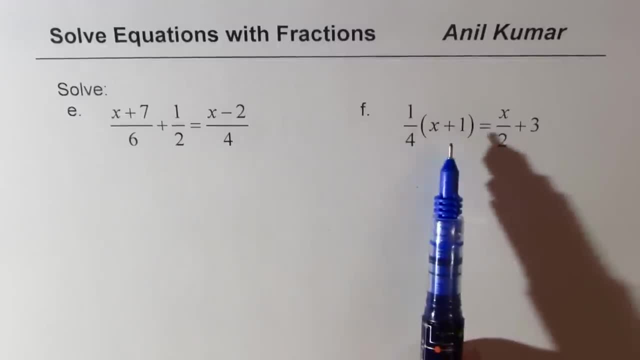 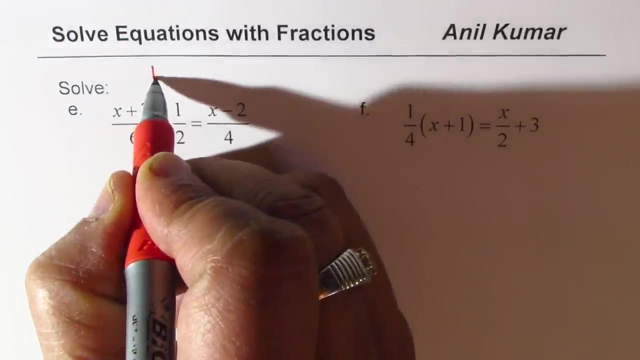 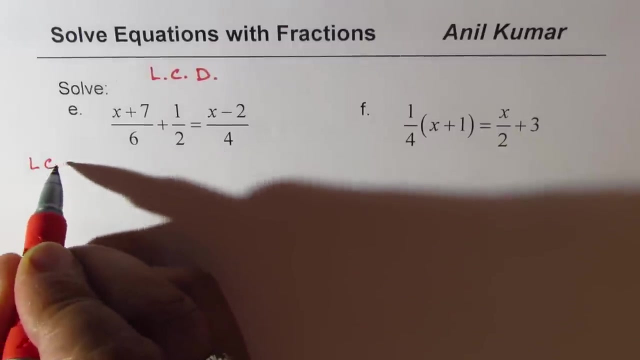 So these two questions. we again have three terms, not just two terms, right? So what do you expect In this case? we have to find the lowest common denominator, right? So let's find lowest common denominator. So lowest common denominator. 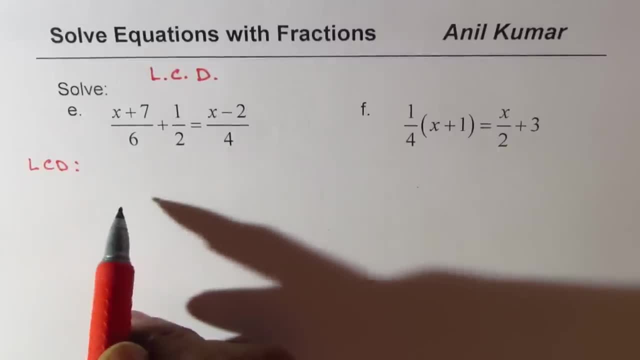 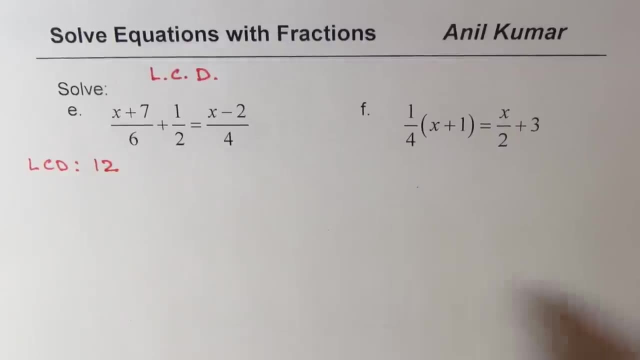 Which, Which is 6,, 2,, 4, is what Is 12, right, So is 12.. Now, for some of you, how do we figure this out? Let's take that now. So, to find this, we have a ladder division method. 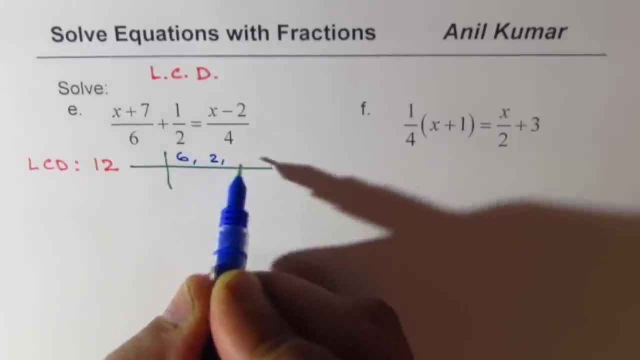 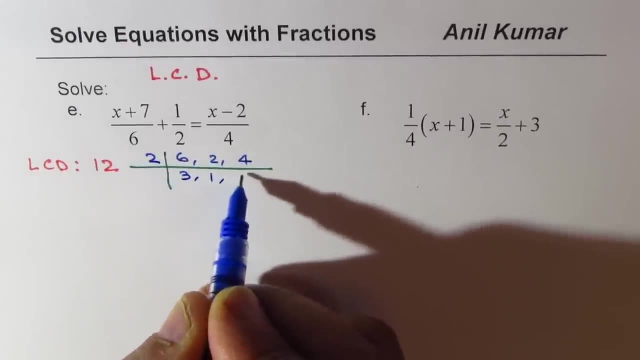 You could write all these numbers 6,, 2, and 4, divided by some common factor, let's say 2. in this case we get 3 times 1 and 2.. So 2 goes 3 times in 6.. 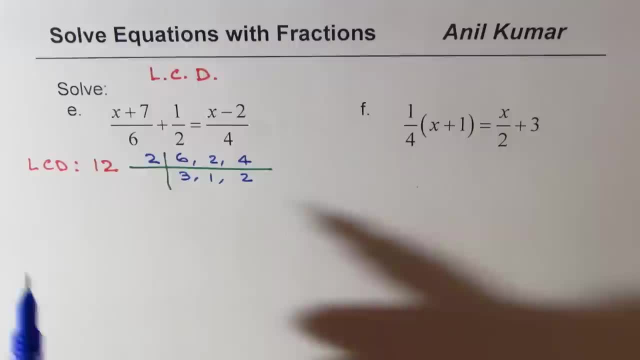 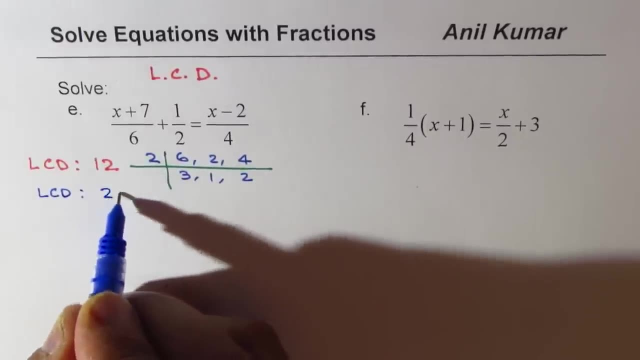 1 times in 2.. 2 times in 4.. So we're left with these numbers. So the lowest common denominator- I should say multiple now, because we found that is 2 times 3 times 1 times 2, which is 12.. 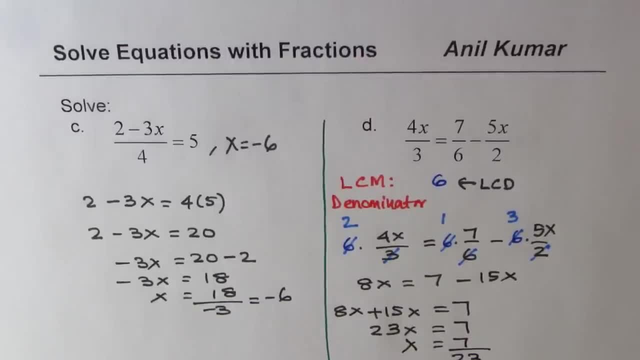 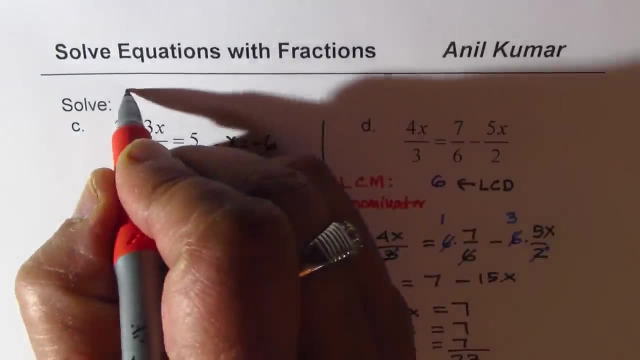 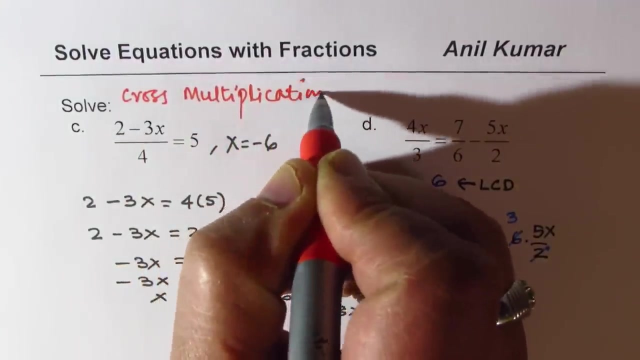 So that becomes the solution for the given equation. So I hope these steps are absolutely clear. So in this page we have seen both the techniques. Here we did cross multiplication And then in D we found the lowest common denominator, which is actually the lowest. 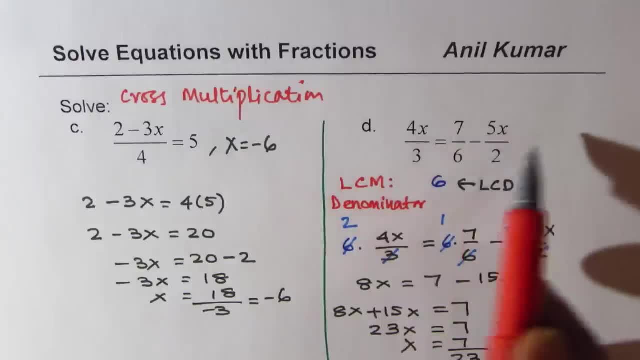 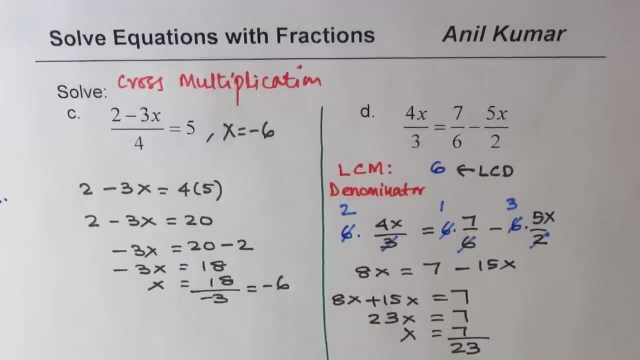 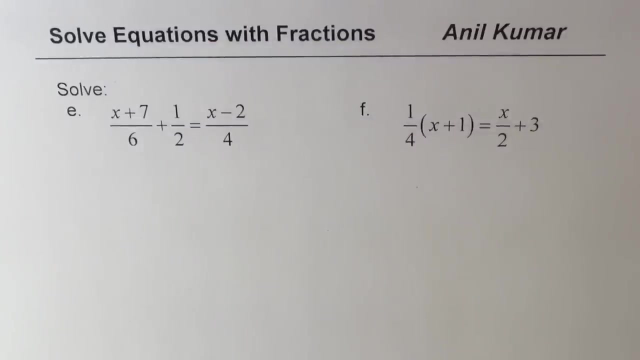 common multiple of the denominators. Multiplying the same gets rid of the denominator And then you can solve as shown here. So I hope the strategy is absolutely clear. Let's move on and take up the rest of the questions. Now I would like you to pause this video, apply the right strategy and then solve. 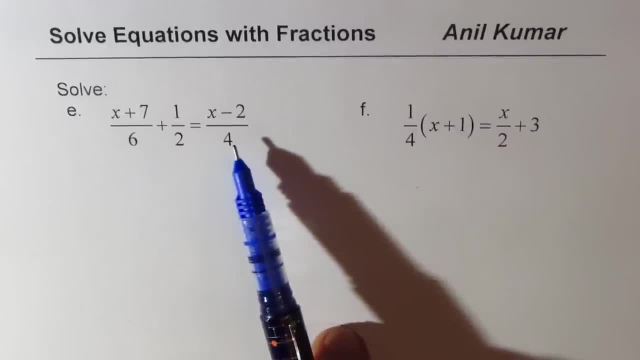 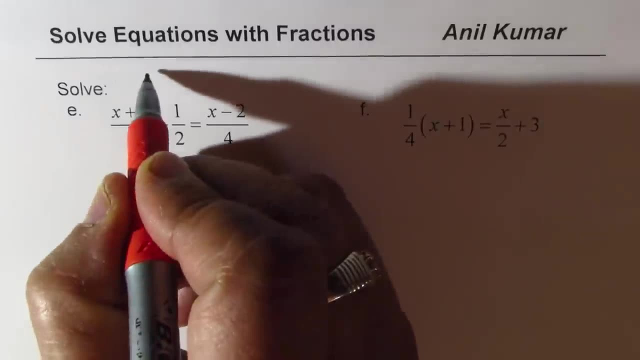 So these two steps are very simple, These two questions. we again have three terms, not just two terms, right? So what do you expect In this case? we have to find the lowest common denominator, right? So let's find lowest common denominator. 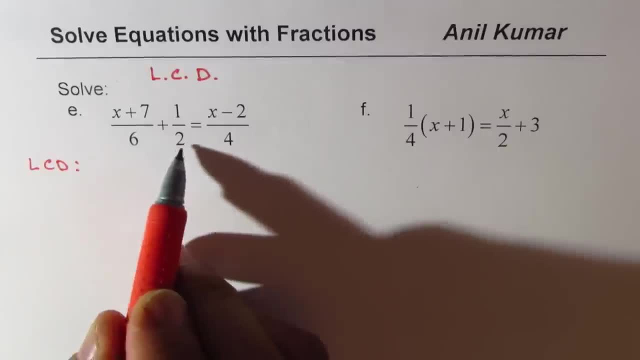 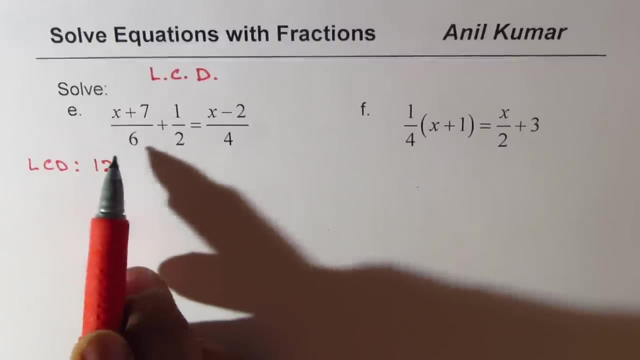 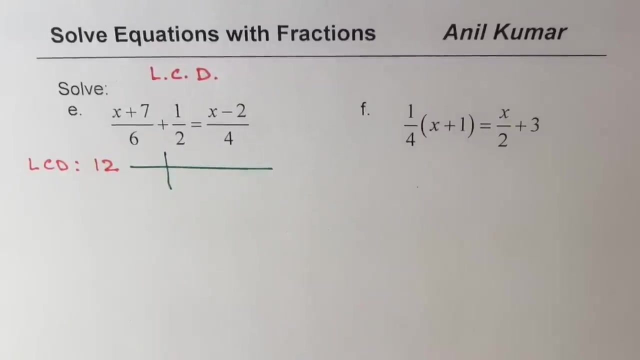 So lowest common denominator, which is 624, is: what Is 12,? right, So is 12.. Now, for some of you, how do we figure this out? Let's take that now. So to find this, we have a ladder division method. 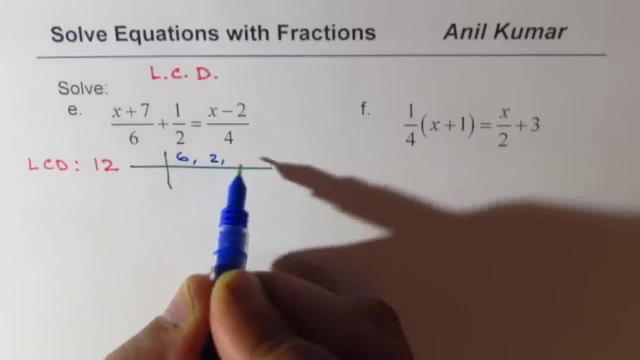 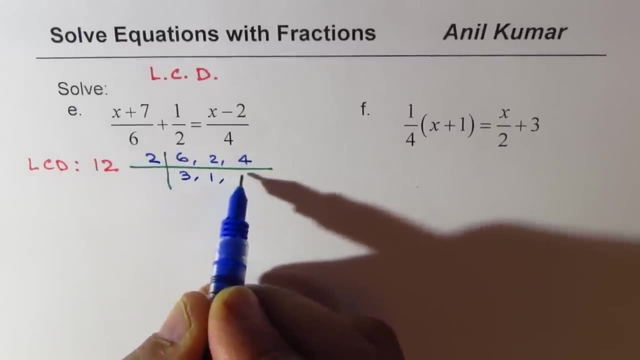 You could write all these numbers- 6,, 2, and 4, divided by some common factor, let's say 2. in this case We get 3 times 1 and 2.. So 2 goes 3 times in 6,, 1 times in 2,, 2 times in 4.. 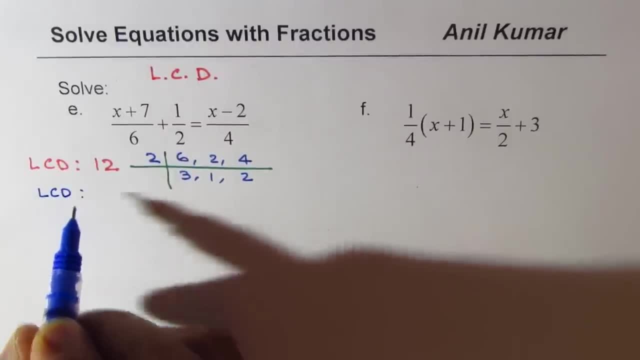 So we're left with these numbers. So the lowest common denominator, I should say multiple now, because we found that is 2 times 3 times 1.. So we're left with these numbers. So the lowest common denominator- I should say multiple now, because we found that is 2 times 3 times 1.. 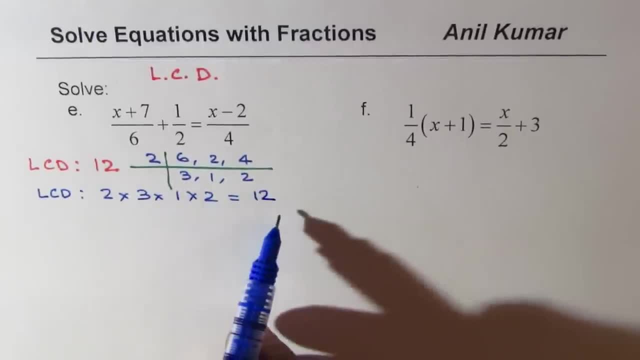 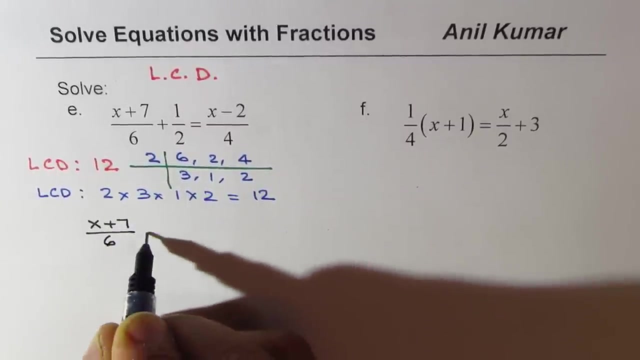 So we have 1 times 2,, which is 12.. So that is the technique of finding the lowest common denominator, Perfect. So once we find that we have to multiply by this number to all the terms, So we have x plus 7, over 6, plus. so we're going to multiply this by 12.. 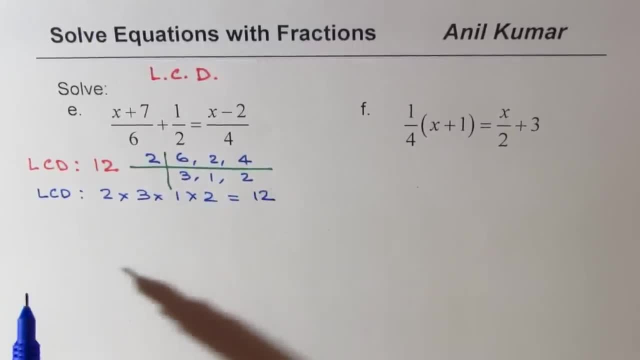 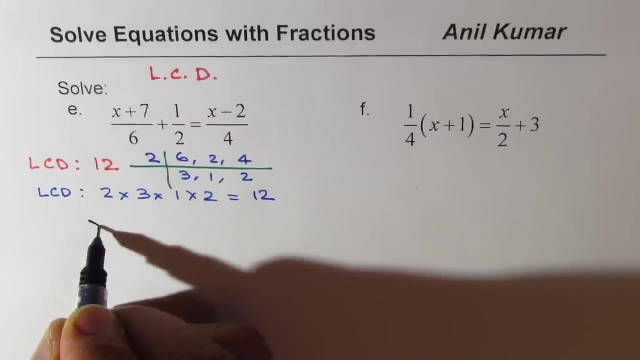 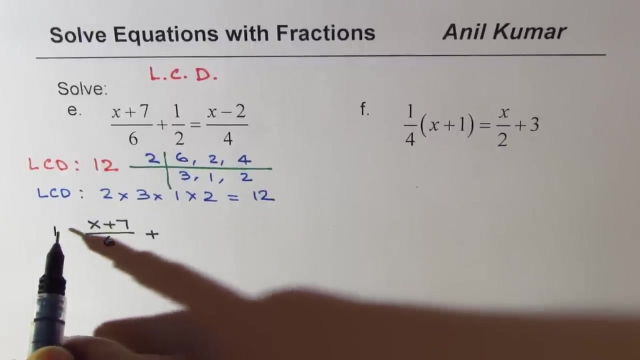 So that is the technique of finding lowest common denominator, perfect. So once we find that we have to multiply by this number to all the terms, So we have x plus 7 over 6 plus 7 over 6. Perfect. So we're going to multiply this by 12.. 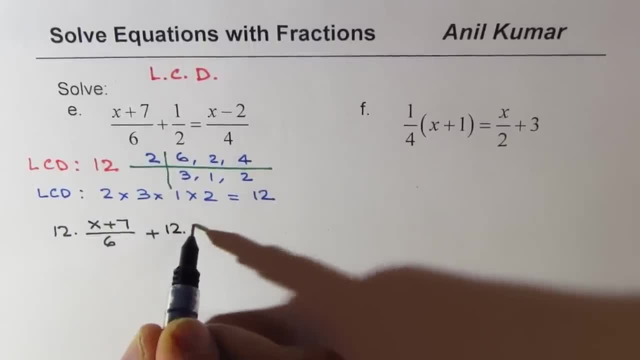 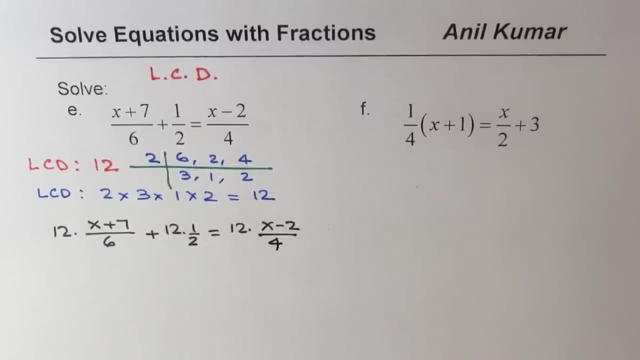 So that is this: 12.. Now, 12 times half equals to 12 times x minus 2 over 4.. As expected, all the denominators can now be cancelled with 12.. So 6 goes 2 times, 2 goes 6 times, 4 goes 3 times. 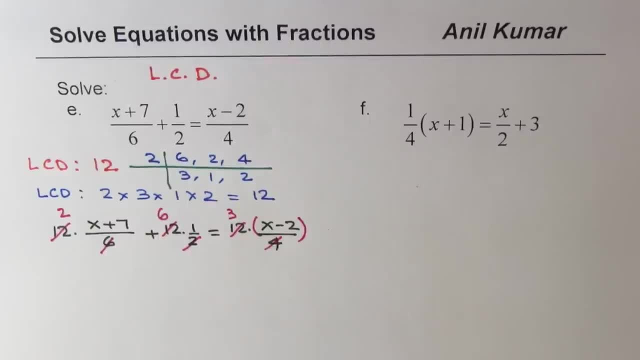 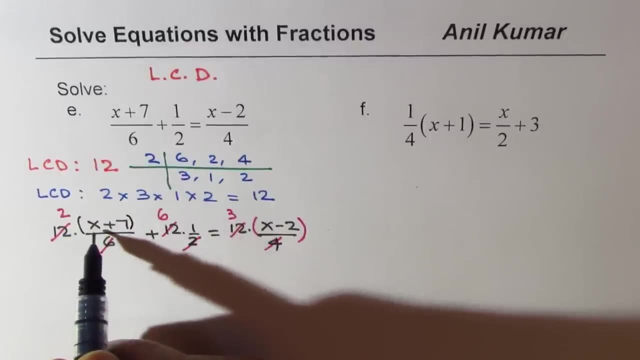 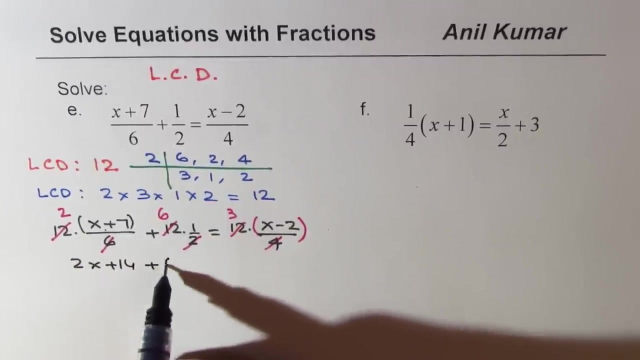 Now this 3 should be multiplied to both. Remember this part, right, Otherwise you will get wrong answer. Same here: 2 has to be multiplied with both x and 7.. So when you open this bracket, you get 2x plus 14. plus 6 equals to 3x minus 6.. 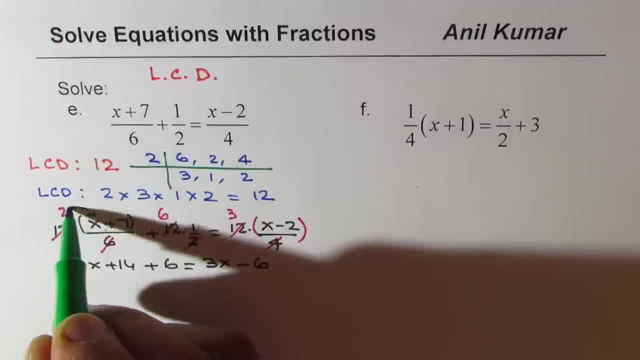 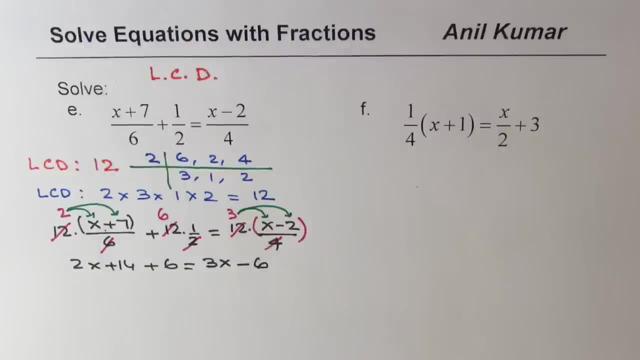 I hope this step is clear. We are multiplying this 2 with both the numbers right. Find the distributive property. Now you have to solve bringing the x terms together and the constants together. Sometimes we know 3x is higher. we'll bring x to the right side. 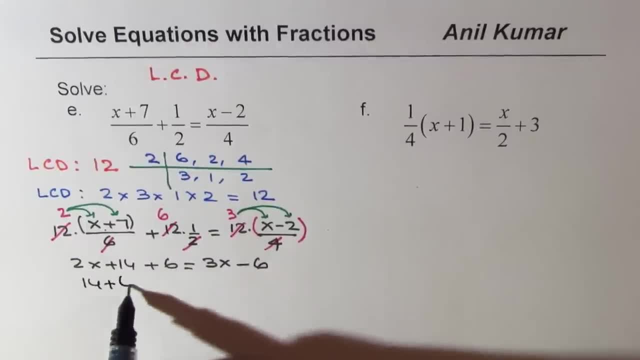 We have 14 plus 6, let me write 14 plus 6.. This 6 coming this side will become a positive 6, 3x minus 2x, so we get x equals to 26.. So x equals to 26 is our answer. 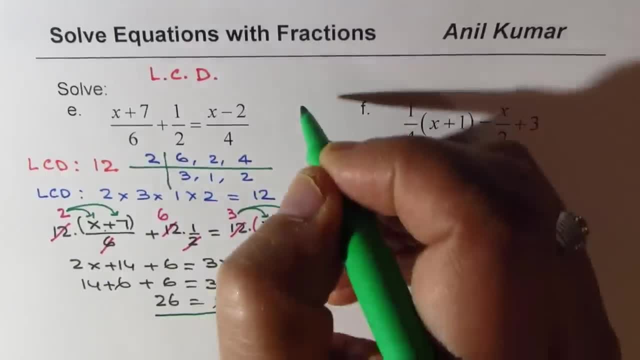 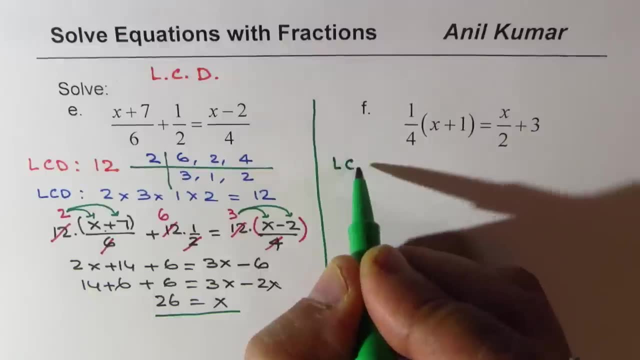 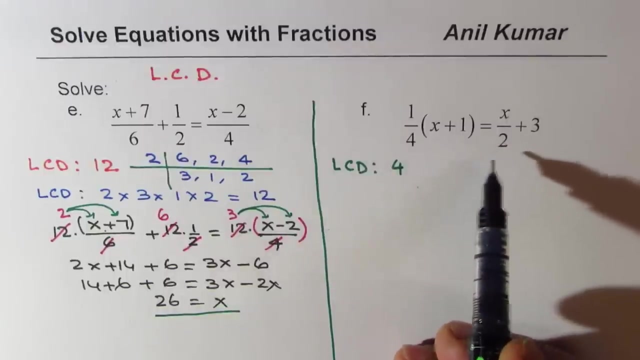 Thank you, Is that clear? Now let's do the next one. So here, what is the lowest common denominator? 4 and 2, it is 4, right, Since 4 is multiple of 2.. So we'll multiply everything by 4.. 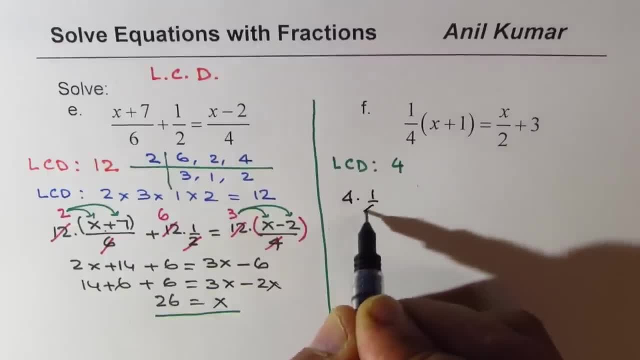 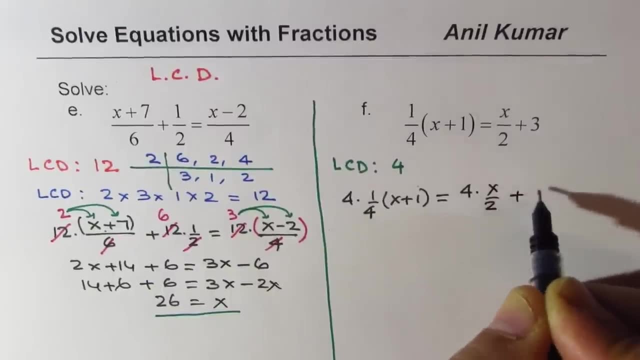 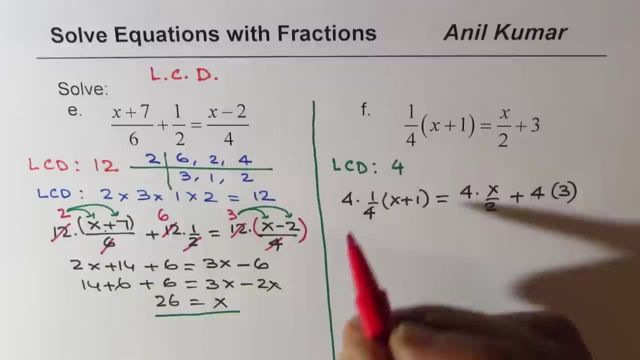 So what do we get? We get 4 times 1 over 4. X plus 1 in brackets equals to 4 times x over 2. Plus 4 times 3.. So here 4 and 4 cancels. 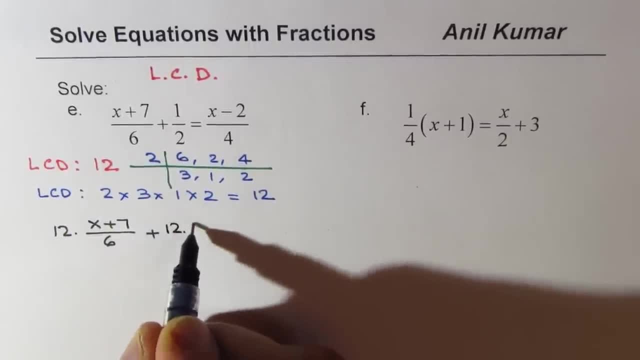 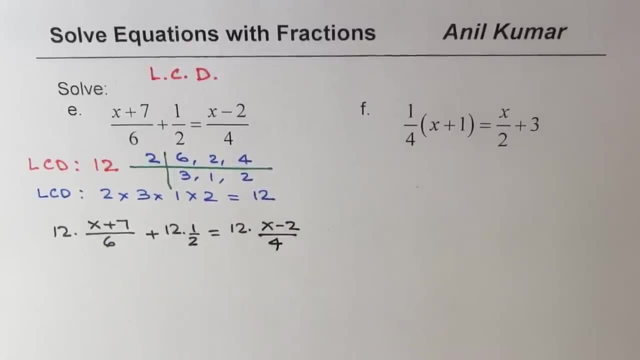 So that is this: 12.. Now, 12 times half equals to 12 times x minus 2. So that is x over 4.. As expected, all the denominators can now be cancelled with 12.. So 6 goes 2 times. 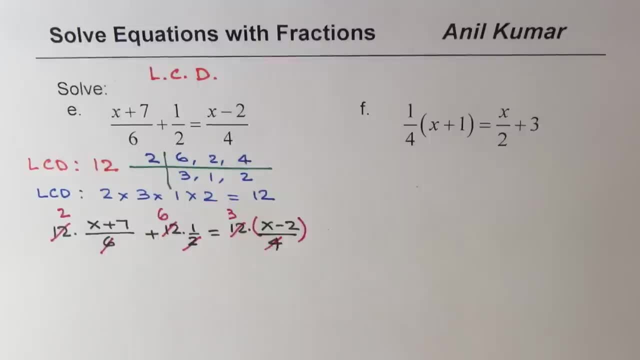 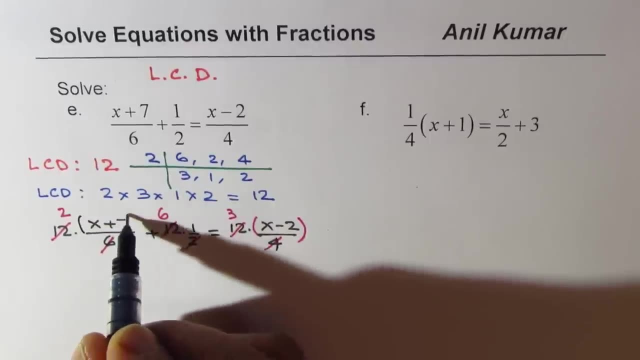 2 goes 6 times, 4 goes 3 times. Now this 3 should be multiplied to both. Remember this part right, Otherwise you will get wrong answer. Same here: 2 has to be multiplied with both x and 7.. 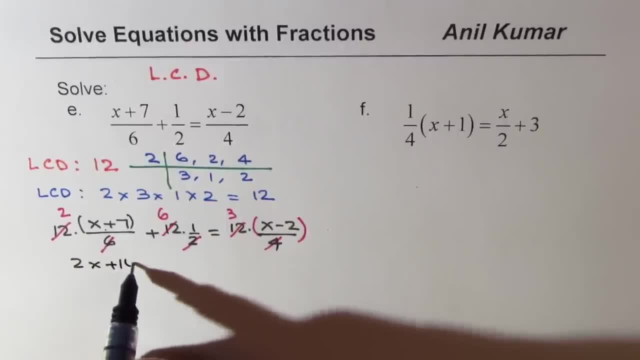 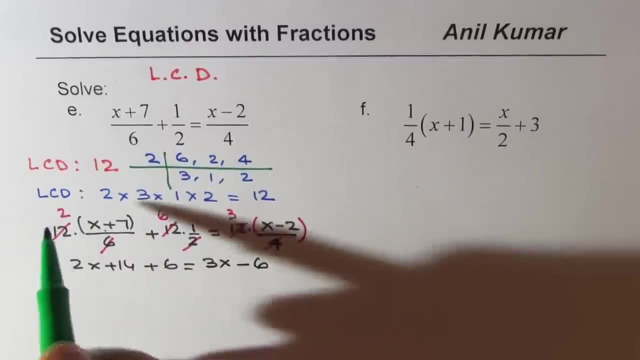 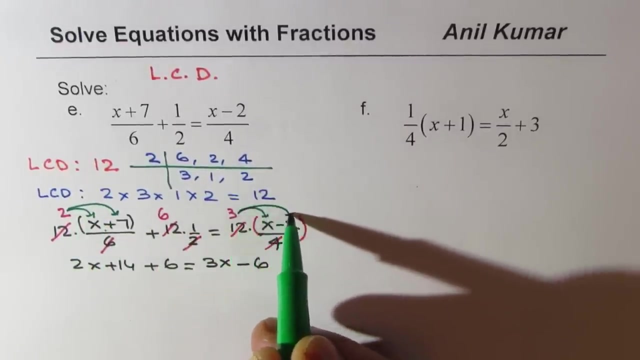 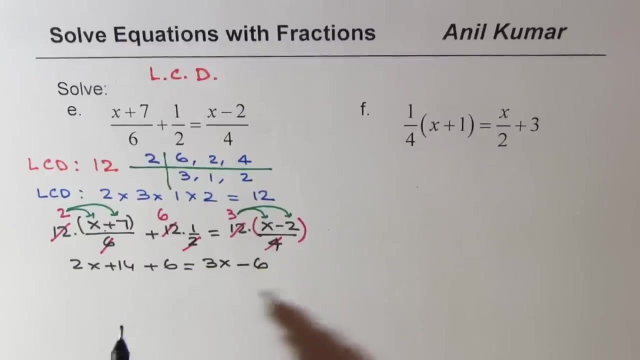 this bracket you get 2x plus 14. plus 6 equals to 3x minus 6. i hope this step is clear. we are multiplying this 2 with both the numbers right, applying the distributive property. now you have to solve bringing the x terms together and the constants together. sometimes we know 3x is higher. 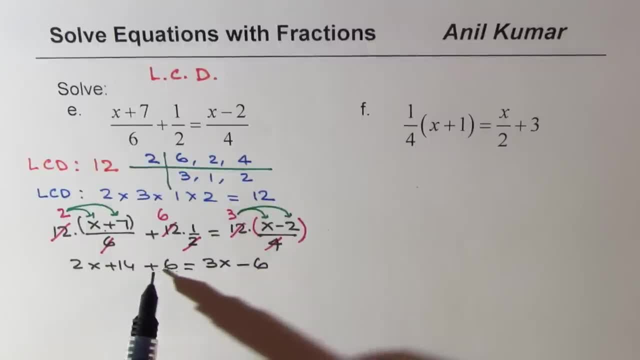 we'll bring x to the right side. we have 14 plus 6. let me write 14 plus 6. this 6 coming this side will become it positive: 6, 3x minus 2x. so we get x equals to 26. so x equals to 26 is our answer. 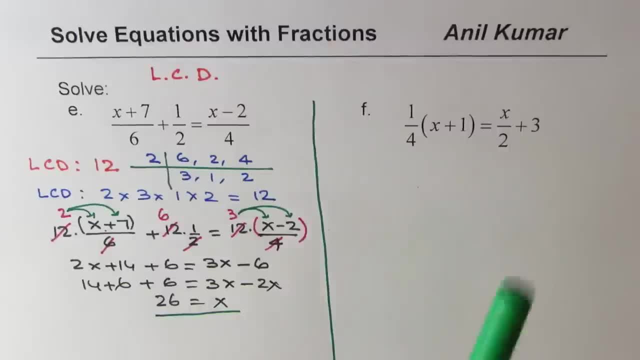 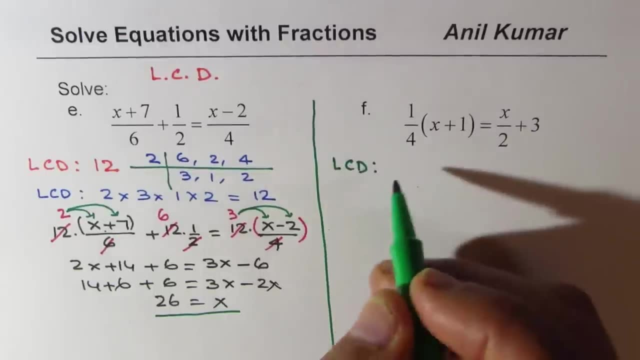 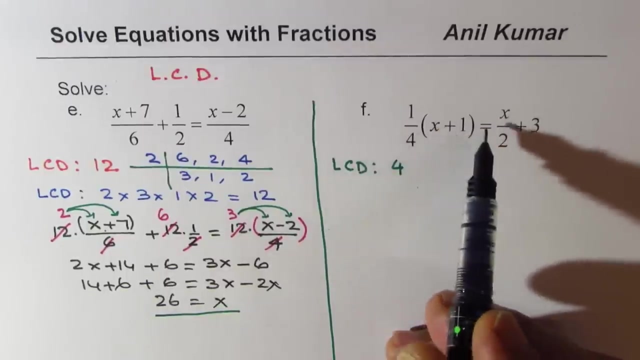 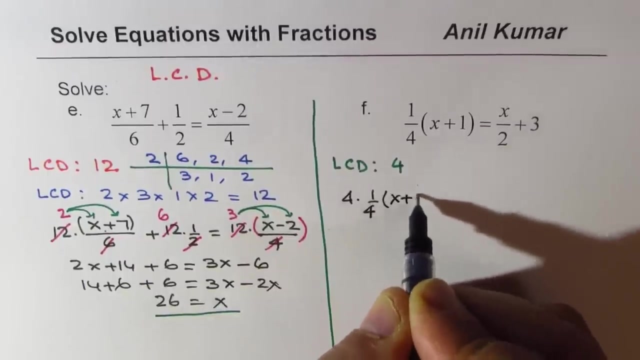 is that clear? now let's do the next one. so here, what is the lowest common denominator? four and two. it is four, right, since four is multiple of two. so we'll multiply everything by four. so what do we get? we get four times one over four x, plus one in brackets. 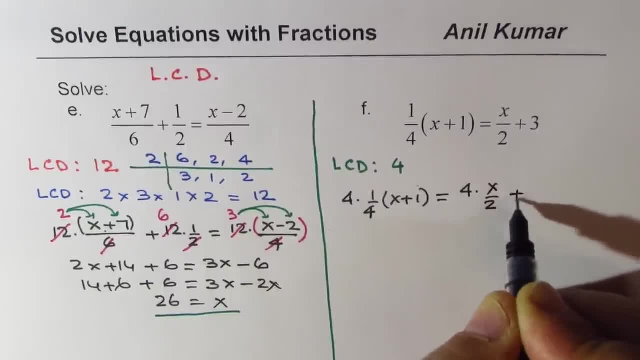 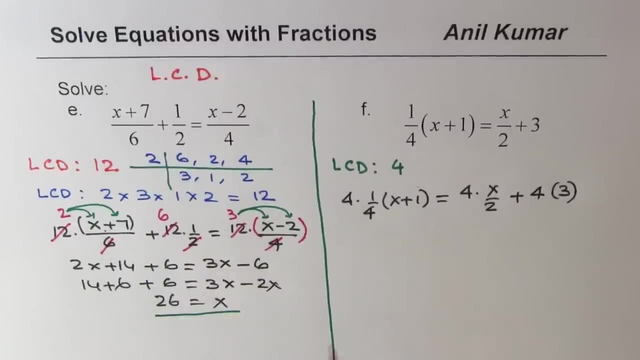 equals to four times x over two plus four times three. so here four and four cancels. in this case we get two times, here it is four times. so when you open the bracket you get x plus one equals to 2x plus 12.. again, i'll take this x to the right side now, since i see that 2x is greater. 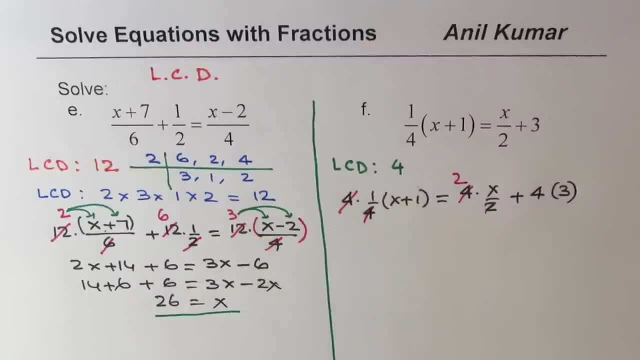 In this case we get 2 times. here it is 4 times. So when you open the bracket you get x plus 1 equals to 2x plus 12.. Again, I'll take this x to the right side now, since I see that 2x is greater. 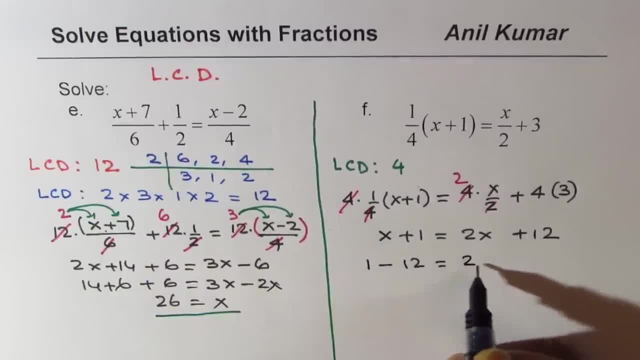 Bring 12 on this side, So we have 1 minus 12.. Equals to 2x minus x. That gives me x equals to minus 11.. So I hope you appreciate this strategy of avoiding the negative sign with x. It also helps, saves time. 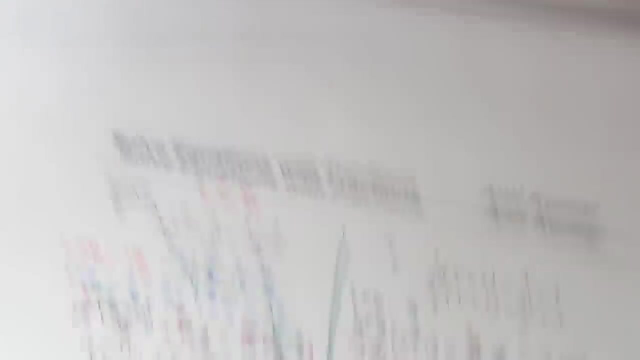 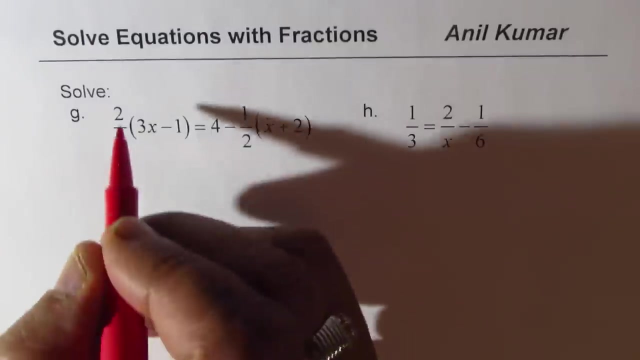 Perfect, Now let's move on and take the last two questions. I hope by now you have learned this strategy. Apply and solve these two questions. Then check with my solution Here: 5 and 2.. So what is the lowest common denominator? 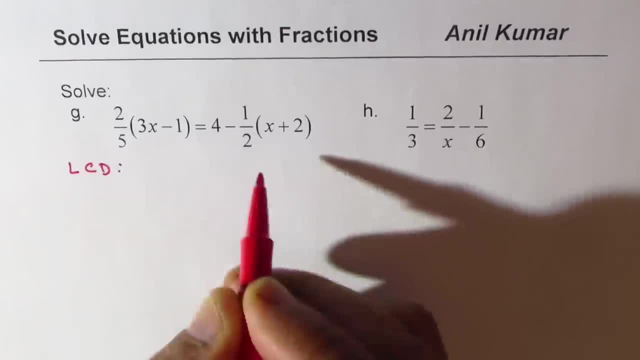 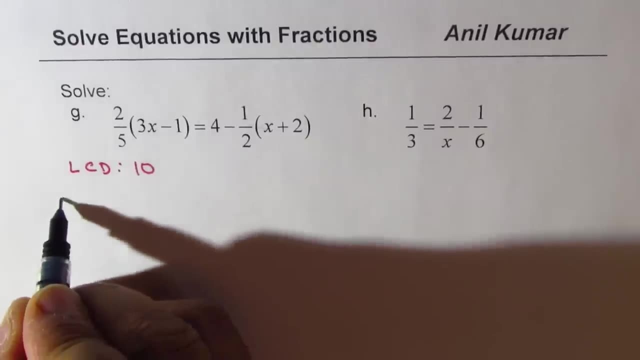 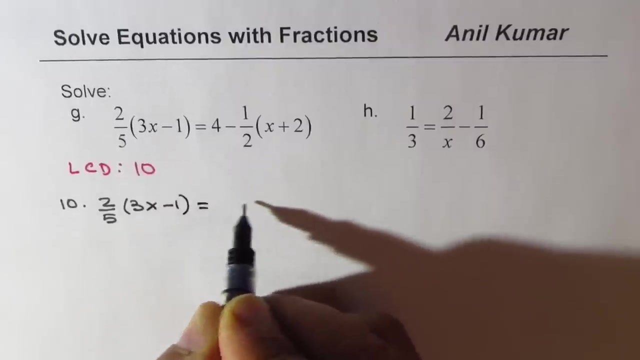 In this case, the lowest common denominator is 10.. So we'll multiply every term by 10.. So what we get here is 10 times 2 over 5 times 3x minus 1 equals to 4 times 10 minus 10 times. 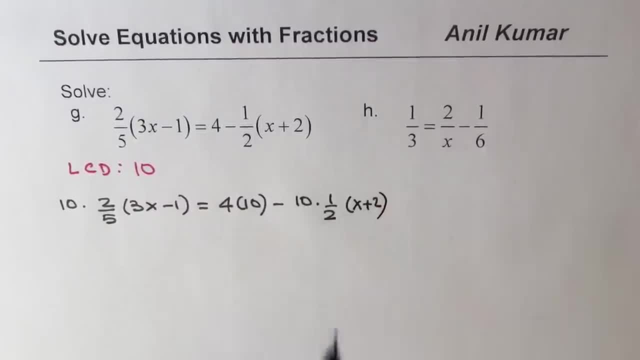 half x plus 2.. Now, when you simplify, 10 goes 2 times with 5 and 5 times with 2.. So 2 times 2 is 4.. So we're at 4 times 3x minus 1 equals to 40 minus. 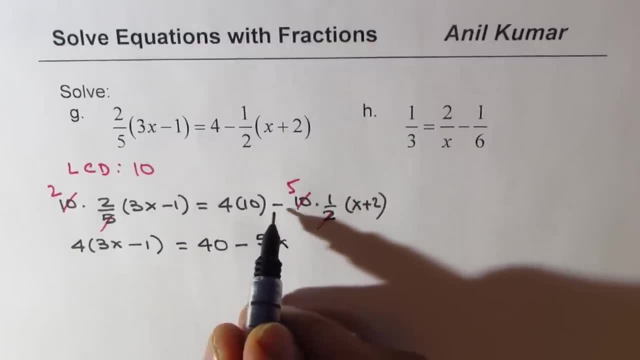 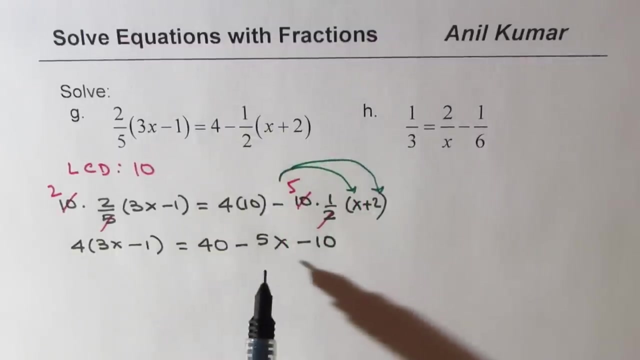 So when you open this bracket, remember to apply minus 5 into both. right, So minus 5x and minus 10.. So take care of minus sign Also. right, So you have to multiply with both the terms. Bring x's together. 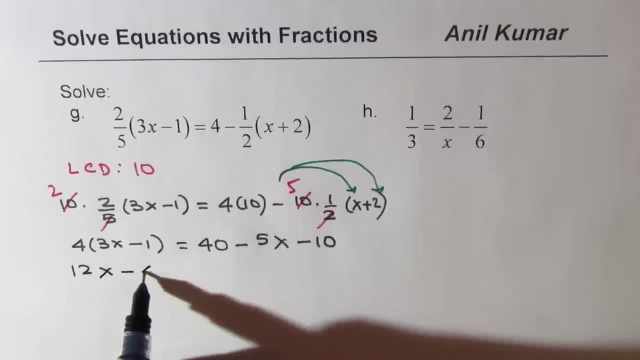 Let's open this bracket also, So we get 12x minus 4 equals to: let's combine them: 40 minus 10 is 30 minus 5x. Bring 5x to the left side. we get 12x plus 5x equals to 30 plus 4, and that is 17x equals. 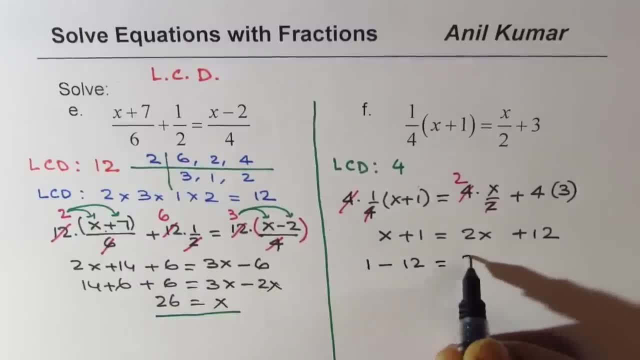 bring 12 on this side, so we have 1 minus 12 equals to 2x minus x. that gives me x equals to minus 11.. so i hope you appreciate this strategy of avoiding the negative sign with x. it also helps, saves time, perfect. now let's move on and take the last two questions. 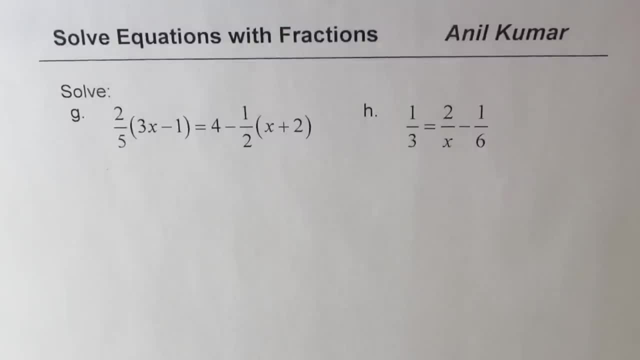 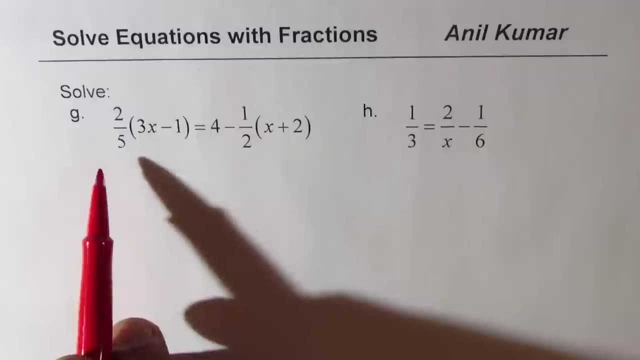 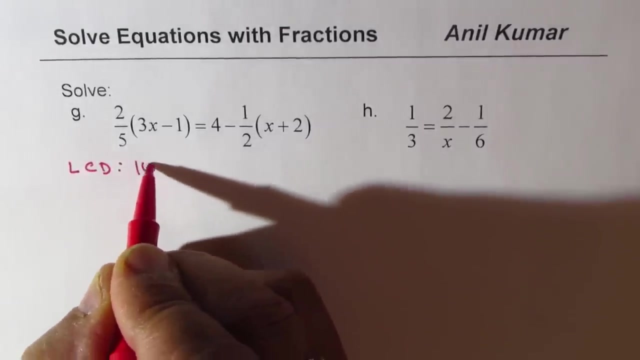 i hope by now you have learned the strategy. apply and solve these two questions. then check with my solution here. five and two. so what is the lowest common denominator? in this case, the lowest common denominator is 10.. so we'll multiply every term by the denominator of the lowest common denominator. 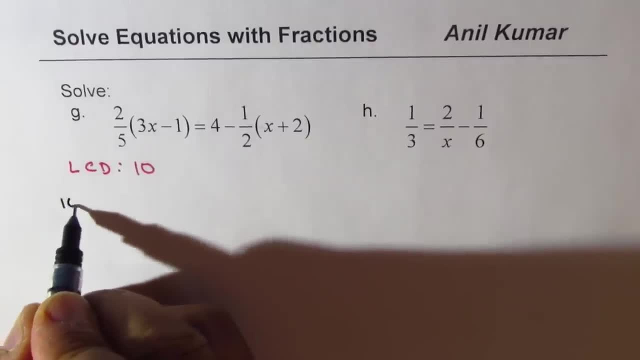 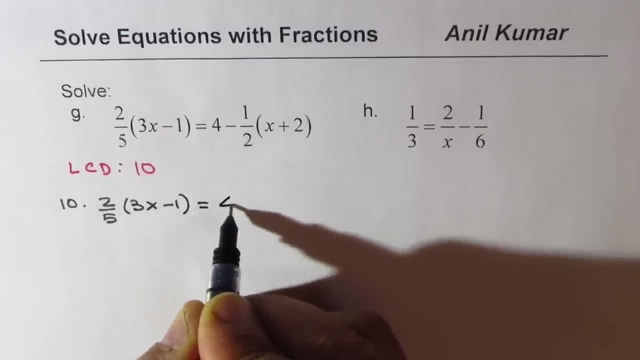 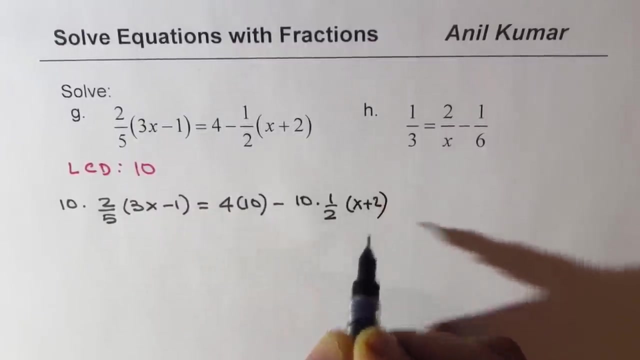 by 10.. so what we get here is 10 times 2 over 5 times 3x minus 1 equals to 4 times 10 minus 10 times half x plus 2.. now, when you simplify, 10 goes two times with five. 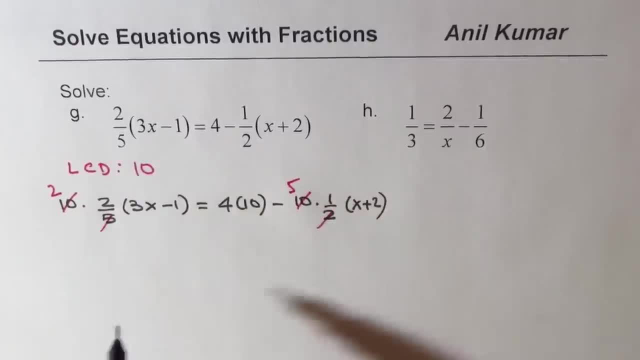 and five times with two. so two times two is four, so we're at four times three. x minus one equals to 40 minus. so when you open this bracket, remember to apply minus 5 into both right. so minus 5, x and minus 10.. so take care of. 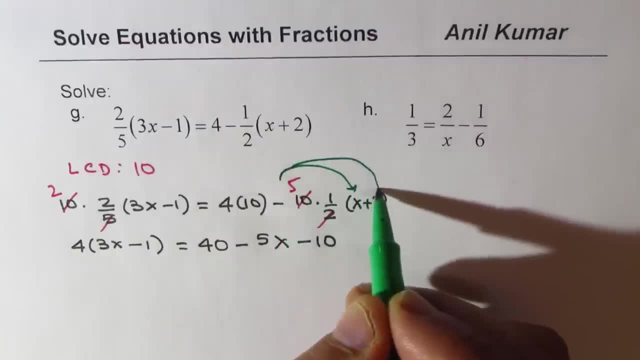 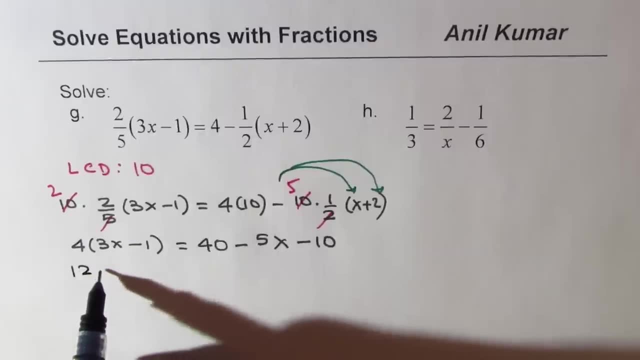 minus sign also right, so you have to multiply with both the terms. bring x's together. let's open this bracket also, so we get 12 x to. let's combine them. 40 minus 10 is 30, minus 5x. Bring 5x to the left side, we get. 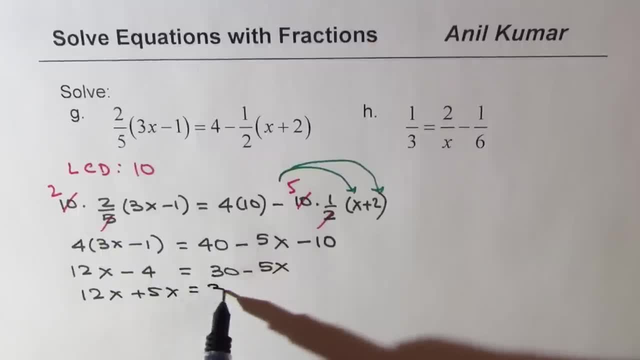 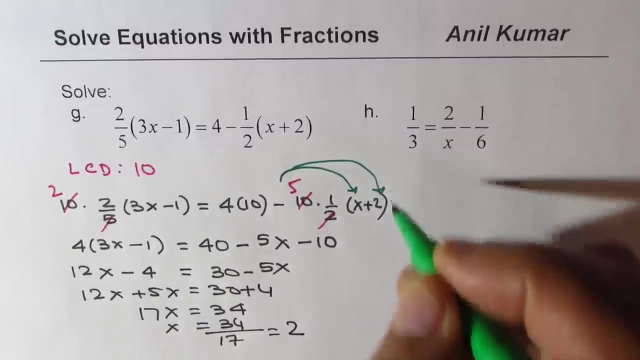 12x plus 5x equals to 30 plus 4, and that is 17x equals to 34, or x is equals to 34 over 17,, which is 2.. Perfect, So that is how you are going to solve it. Now let's take 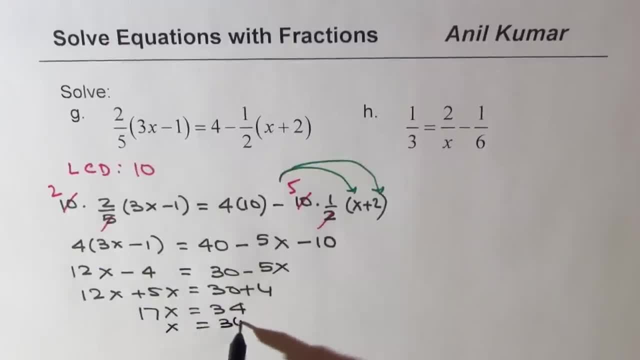 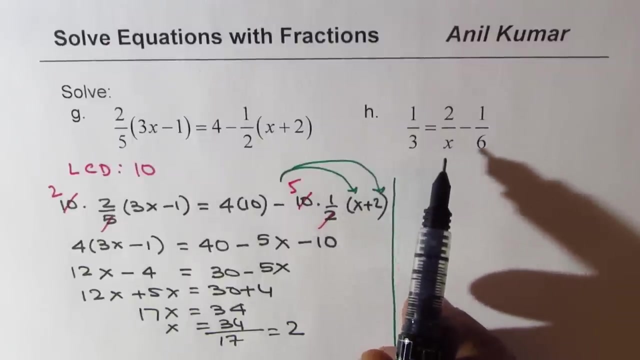 to 34.. Or x is equal to 34 over 17,, which is 2.. Perfect. So that is how you're going to solve it. Now let's take the last example. This is kind of different, since you have x in the denominator. 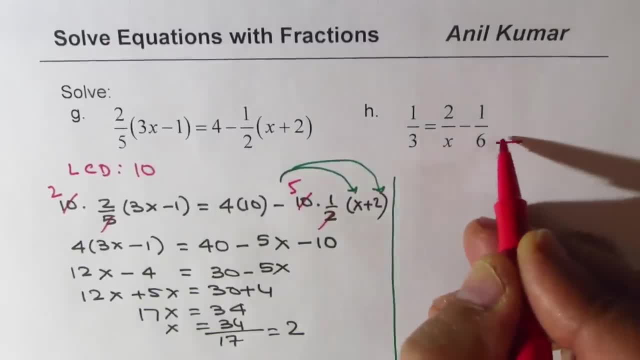 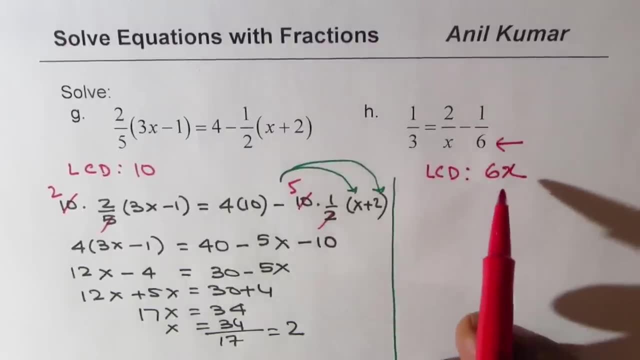 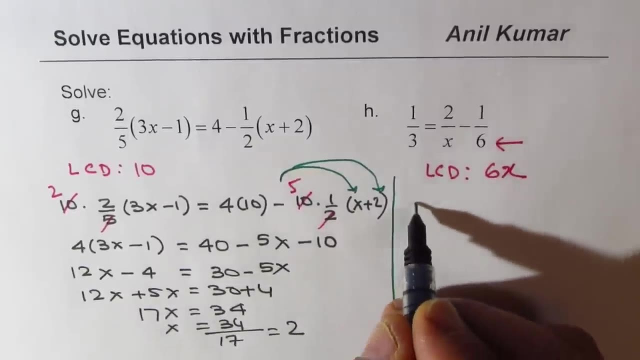 Do you see this? part X is in the denominator. So in this case, what is the lowest common denominator? It is 6x. Do you see that? Not just 6. 6x. So we are going to multiply each term by 6x. 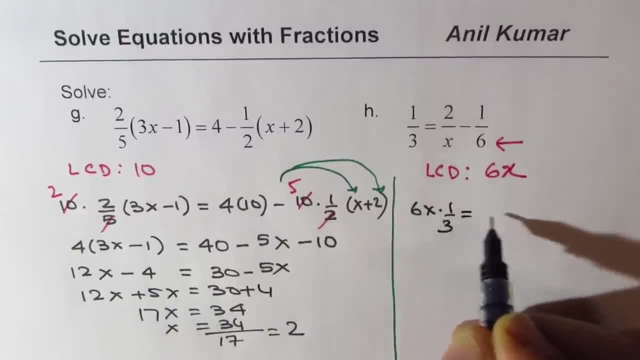 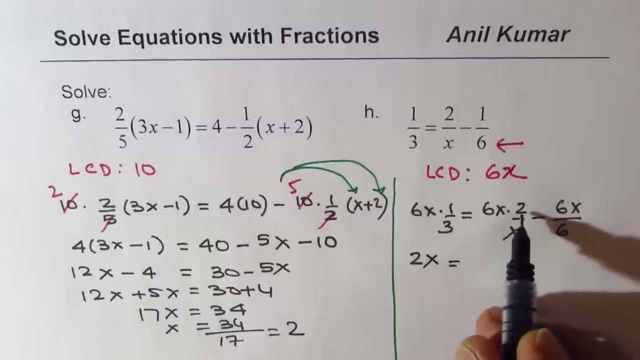 So we have 6x times 1 over 3 equals to 6x times 2 over x, minus 6x over 6. So that gives you 6 divided by 3 is 2.. So we get 2x equals to 6 times 2 is 12.. 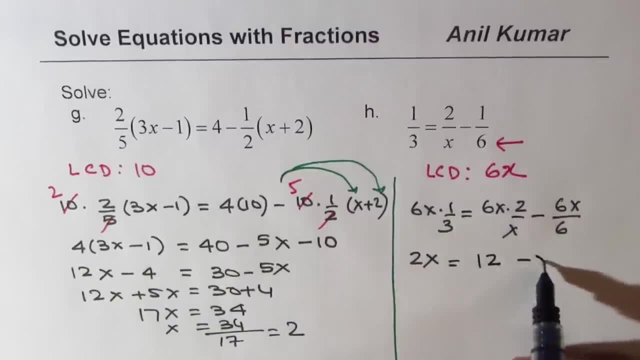 X and x cancel, Right, So we get 12.. And here we get minus x. So see what happens: X and x cancels, This goes 2 times, And 6 and 6 cancel. So we get our equation, which is: 2x equals to 12 minus x. 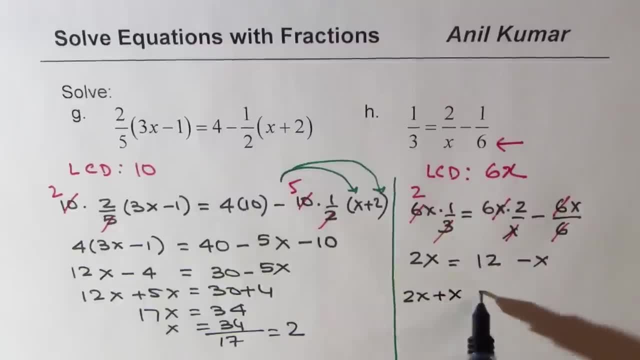 Now bringing x to the left, we have 2x plus x equals to 12,, 3x equals to 12, x is equal to 12 over 3, which is 4.. So I hope the solutions are absolutely clear. 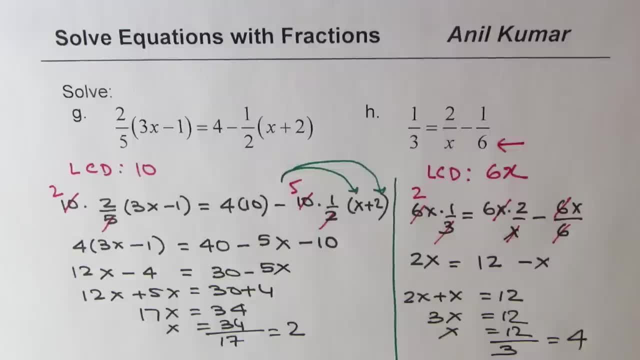 Thank you, That is how it should be solved. Go through these examples once again. So we have different types of strategies applied And these are sufficient to answer or solve any equation involving fractions. Feel free to write your comments and share your views. 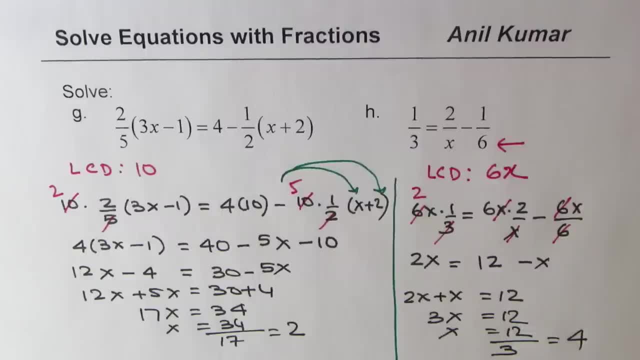 If you really like and subscribe to my videos, that would be great. Thanks for watching and all the best. 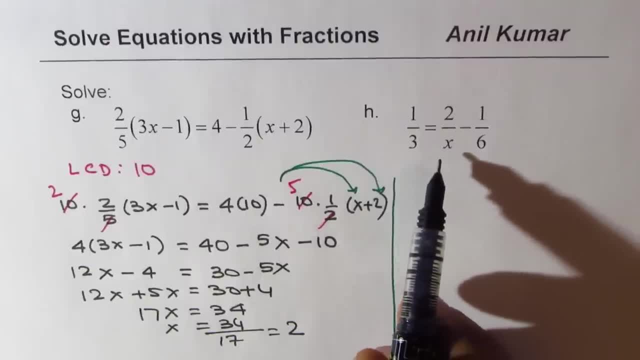 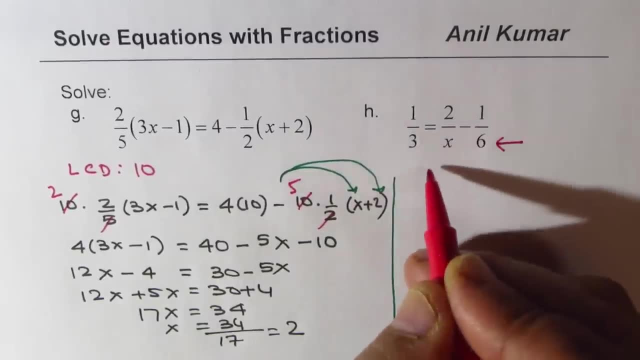 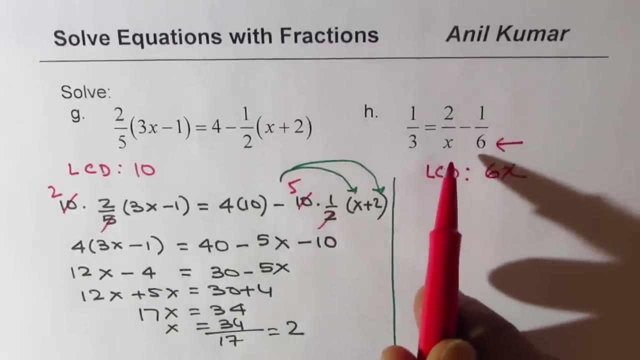 the last example. This is kind of different, since you have x in the denominator. Do you see this part? x is in the denominator. So in this case, what is the lowest common denominator? It is 6x. Do you see that? Not just 6, 6x? So we are going to multiply each term by 6x. 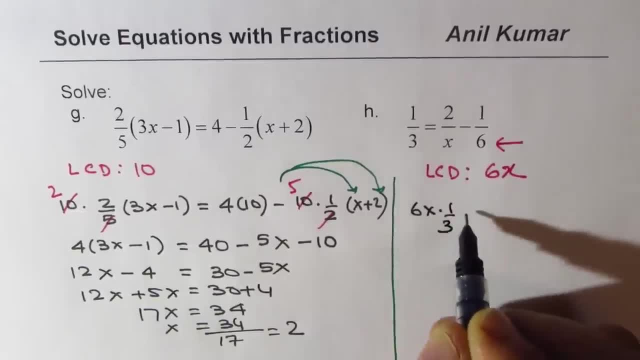 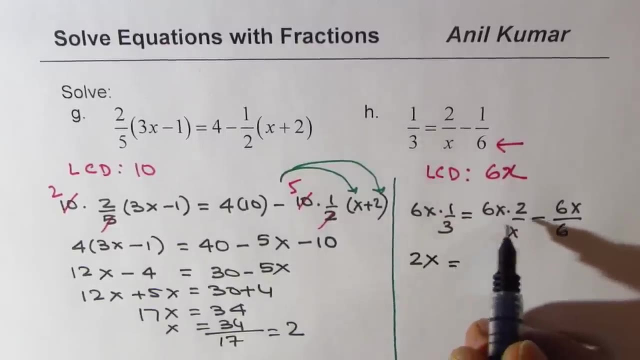 So we have 6x times 1 over 3 equals to 6x times 2 over x Minus 6x over 6. So that gives you 6 divided by 3 is 2.. So we get 2x equals to 6 times 2. 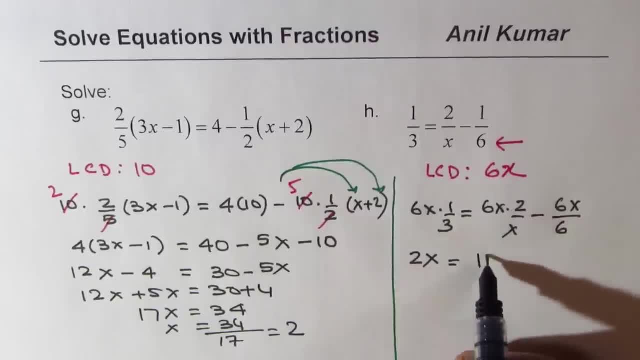 is 12.. x and x cancel, right, So we get 12, and here we get minus x. So see what happens: x and x cancels. This goes 2 times, and 6 and 6 cancel, So we get our equation which: 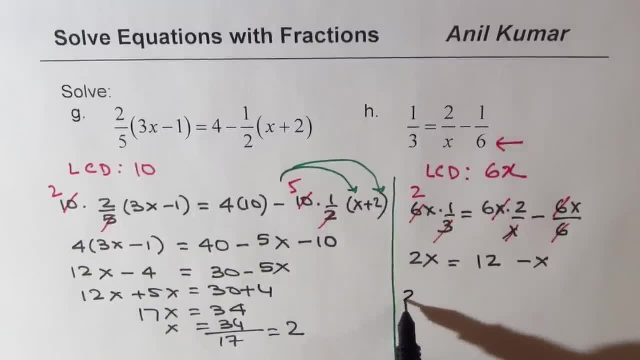 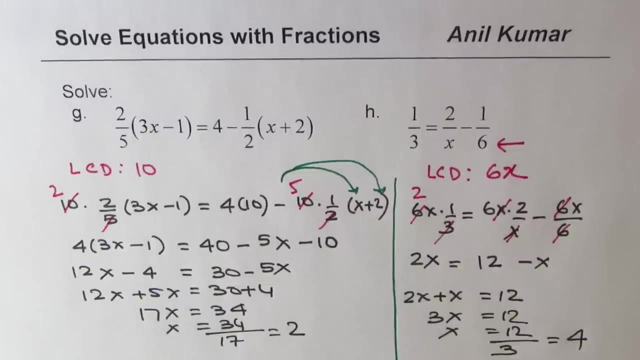 is 12 minus x. Now, bringing x to the left, we have 2x plus x equals to 12.. 3x equals to 12.. x is equals to 12 over 3,, which is 4.. So I hope the solutions are absolutely. 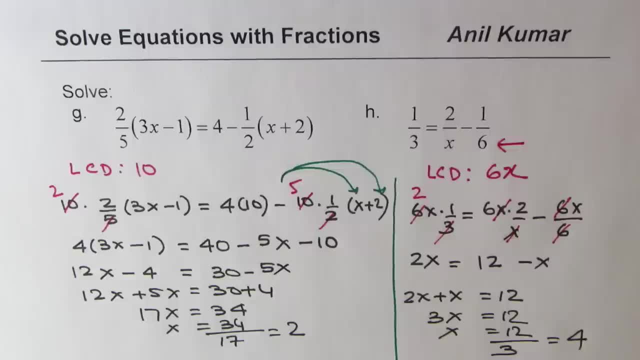 clear. That is how it should be solved. Go through these examples once again. So we have different types of strategies applied and these are sufficient to answer or solve a any equation involving fractions. Feel free to write your comments and share your views. 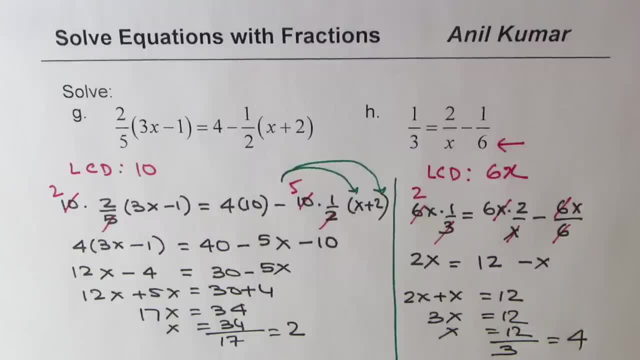 If you really like and subscribe to my videos, that would be great. Thanks for watching and all the best. 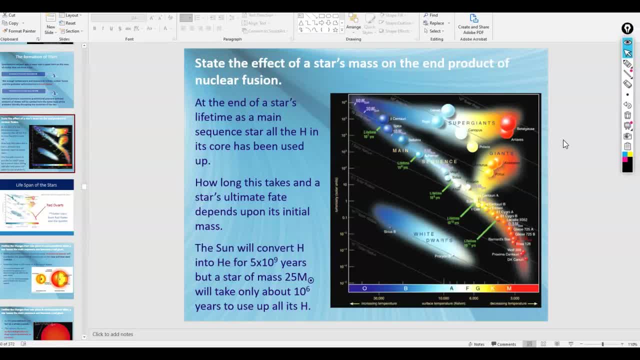 Okay, so in this video we're going to talk a little bit more about stellar evolution, specifically what could happen to a star at the end of its lifetime, depending on the mass of the star. Okay and so in the last video we kind of talked about the formation of stars, we talked about protostars.